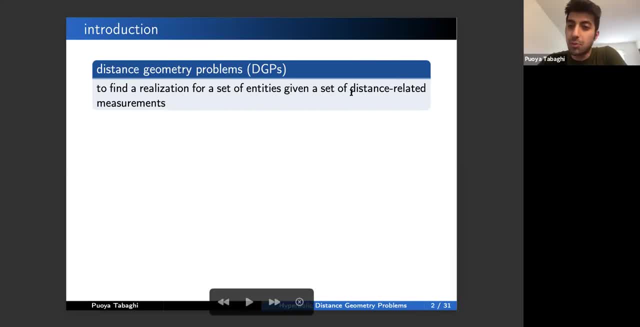 set of distance-related measurements. I use the word distance-related because not always we have exact distances or distances. In some applications- actually many applications- we have dissimilarity data that are different from distance measurements, and I will get to them later on. But from here on I keep talking about dissimilarities. You can in your mind 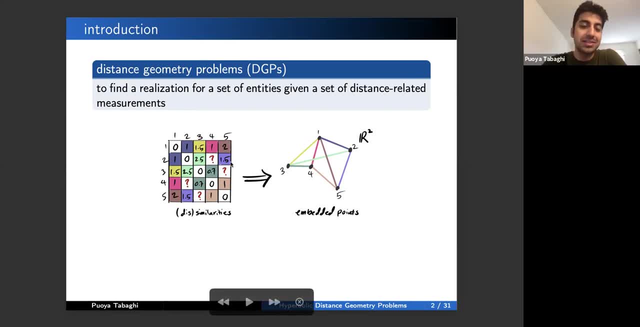 place it with distances. Okay. so here's an example of a DGP For a set of five entities. in an application, you can have a set of dissimilarity or similarity measurements between these pairs of points, and you might have some missing measurements here as well. 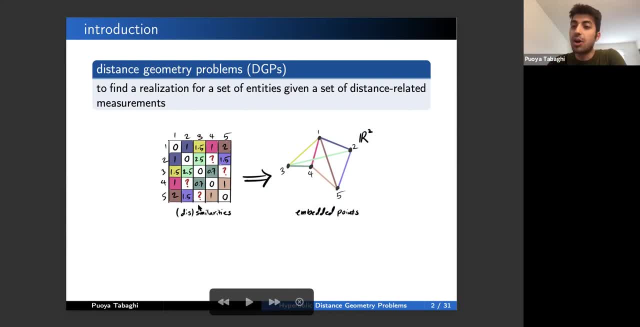 And the goal is to find a realization, for instance in R2, that best represents these measurements. So if the dissimilarities are, for instance, Euclidean distances, then you can think of multi-dimensional scaling, PCA and other variants of metric DGPs as solvers or as variants of 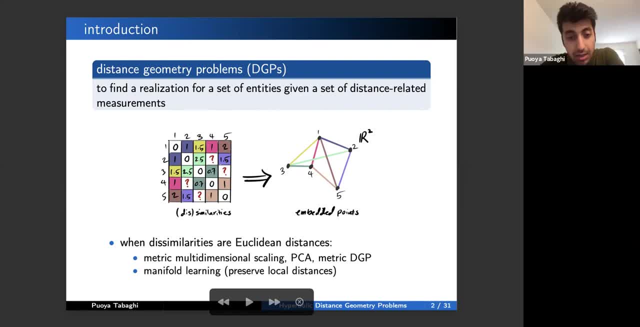 DGPs. Another line of work that kind of related to distance geometry problems are manifold learning problems where we have the distances between pairs of points but we only focus on local distances or the distances within some neighborhood of an entity, and we would like to find an embedding, a low-dimensional embedding, that captures this local geometry of data points. 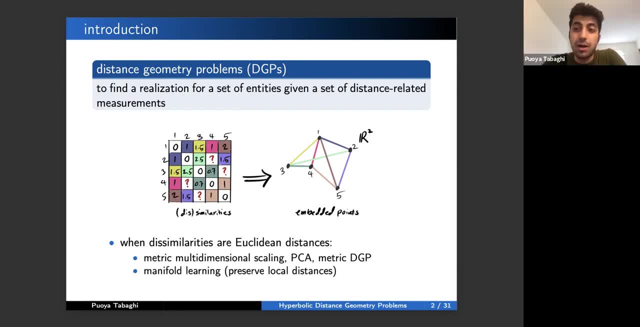 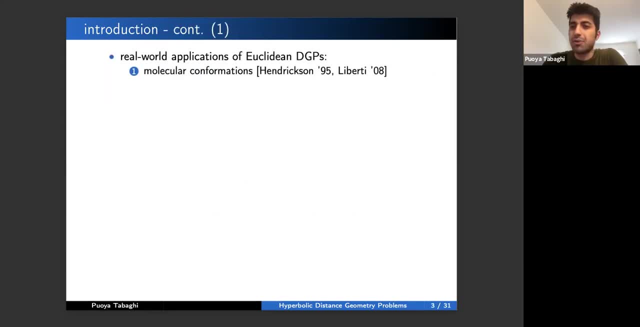 So in a sense even manifold learning problems could be an instance of distance geometry problems. So we've already covered many applications of Euclidean DGPs, so I just rehashed them again. One application could be molecular conformation, where we have nuclear magnetic resonance data and we transform them into distances between atoms and we try to 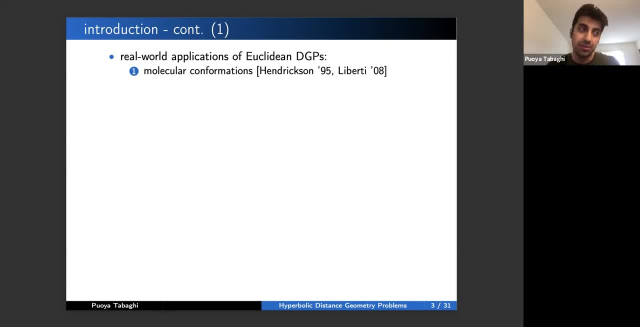 solve DGP. we try to find the molecular structure that realizes this data. This is an instance of unassigned distance geometry problems where we don't know basically which pairs these distances are related to pairs of points. Another application would be sensor network localization where we have signals. 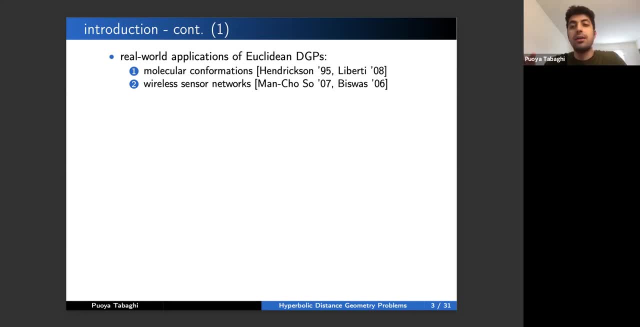 their restraints or their time of arrival and we transform them into distances between nodes And the goal is to estimate the topology of the network Or one application. other application could be robotics, where we have robot, robot swarms, lots of robots, and these robots get to communicate with each other, being neighboring. 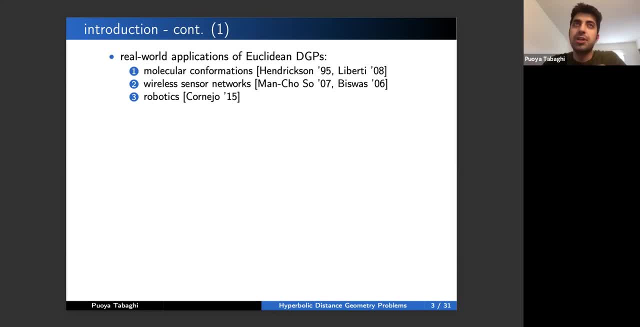 robots and share distance information, but we don't have the global distance information and we want to localize all of these robots at the same time. so these are real world applications of dgps where the data points belong into r2 or r3. but that's not the end of the story. we might have 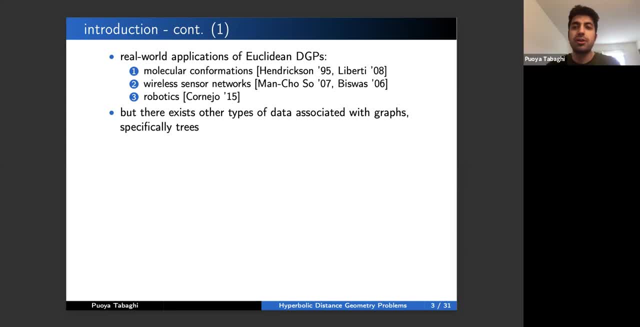 other types of data that usually are associated with graphs, and especially here we are talking about trees, and you can- you can think about it as having an underlying tree, which you may not even know about, but you can think about this as a tree and you can think about it as a tree, and 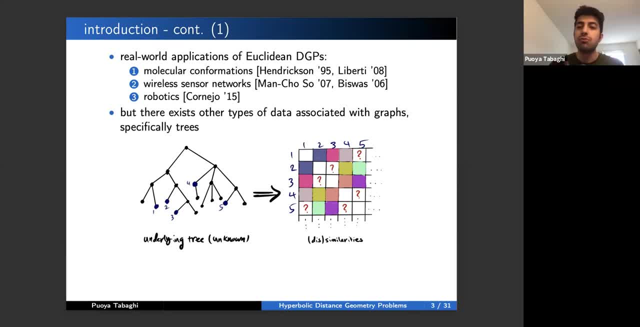 can think about it as having an underlying tree which you may not even know about, but you can know what that tree is. but you have reasons to believe that there is a tree And you get to see similarity or dissimilarity of scores between a set of entities or nodes on that tree. 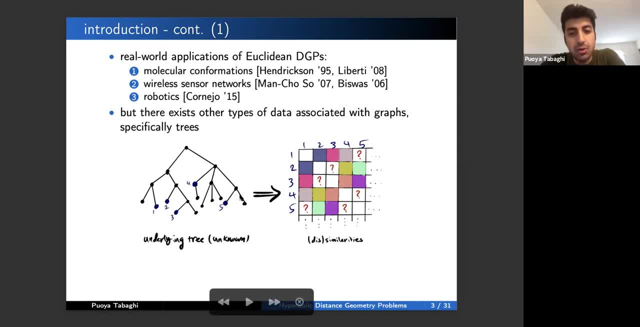 And these dissimilarities are generated via a function of distances on the tree that are defined on the tree. So here, if you have similarity scores like this, then it's not obvious that Euclidean representation for this tree could be optimal. As a matter of fact, I will show that. 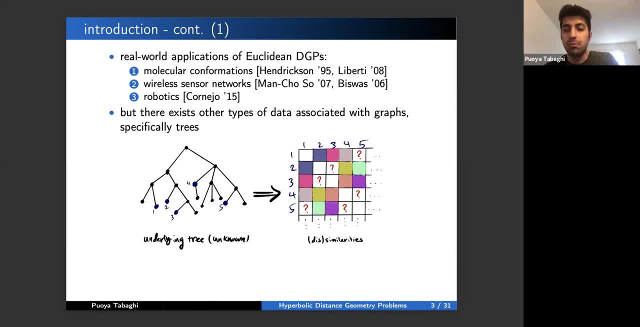 it wouldn't be and we have to go about embedding such dissimilarity measurements In hyperbolic spaces. And such data can be found in many domains. For instance, you can think about taxonomies in biology, where we have a different species And we know that there is an underlying 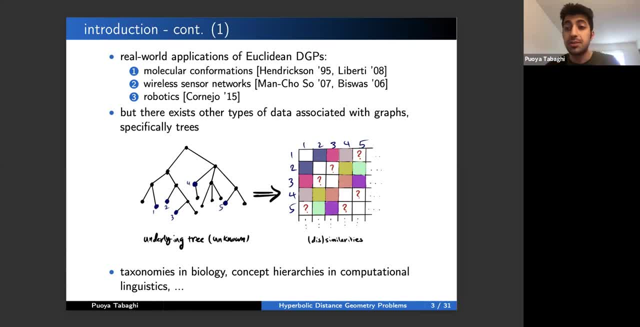 tree that explains the different categories of these species, And so if you want to find a representation and visualize this taxonomy, then we're talking about embedding a tree Or another application would be concept hierarchies in computational linguistics, where we have 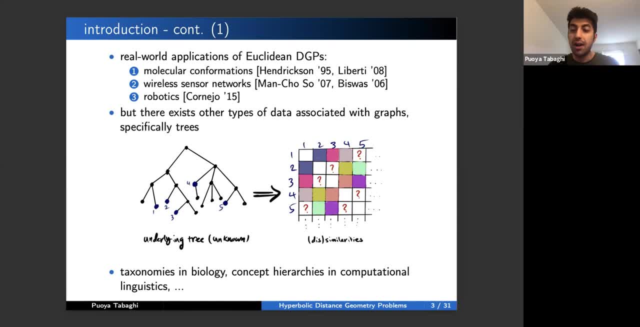 for instance, words that they have semantic hierarchies between each other, And if you want to embed these words and find the vector representation for these words, then we want to leverage these hierarchies so that we get a better, more meaningful embedding for them. 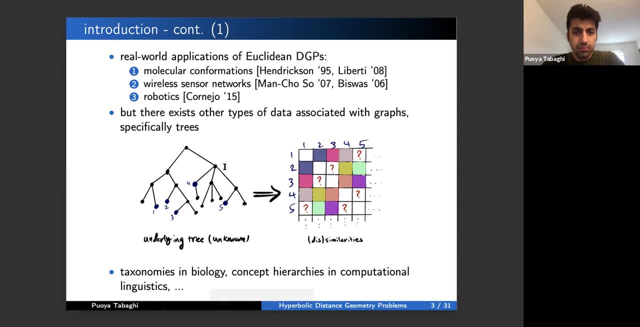 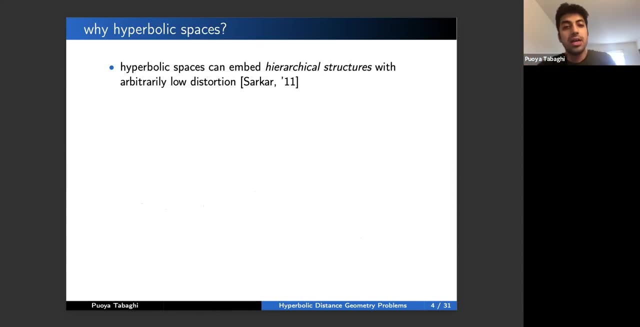 and subsequently perform different tasks- natural language processing tasks- more efficiently. So why are we considering hyperbolic spaces? Well, in 2011,, Sarkar showed that hyperbolic spaces can embed hierarchical structures, or, more specifically, weighted trees with arbitrary load distortion, And this was in just 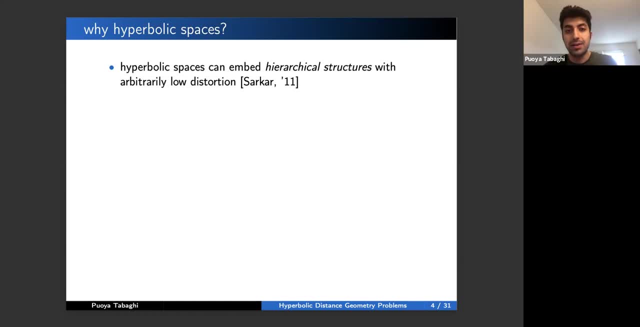 two-dimensional hyperbolic spaces. So we can embed hyperbolic structures And we can embed hierarchical space, And the distortion was up to a multiplicative scaler. but for most applications that doesn't really matter for us, And so one kind of simple way of thinking about it. 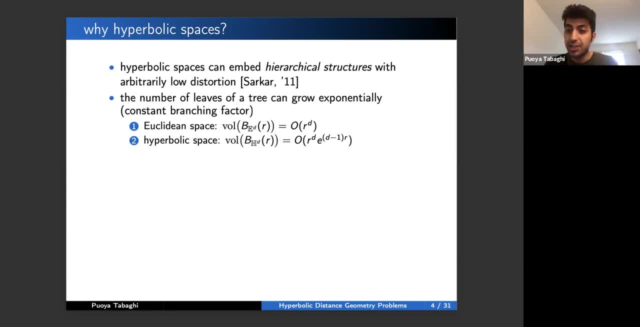 is that you can think about a tree that is growing, whose depth is growing. So the number of leaves, if you have constant branching factor, would grow exponentially. And if you want to embed this tree in Euclidean space, we better be able to have enough space, basically. 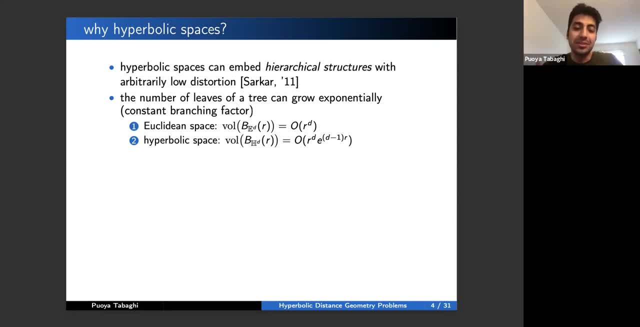 to embed this tree And simple reasoning basically says we don't have enough space because the radius of a ball in Euclidean space grows polynomially, not exponentially. in Euclidean space with dimension, sorry with radius, But in hyperbolic space this volume grows. 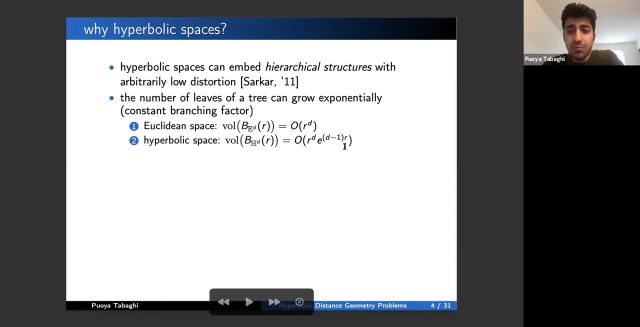 exponentially, even for two-dimensional. So in a sense hyperbolic space is a little bit more roomier to embed tree-like structures. And here I did a real simple experiment: I generated one specific tree weighted tree and I embed them in a tree And I put them in a tree, and I put them in a tree and I 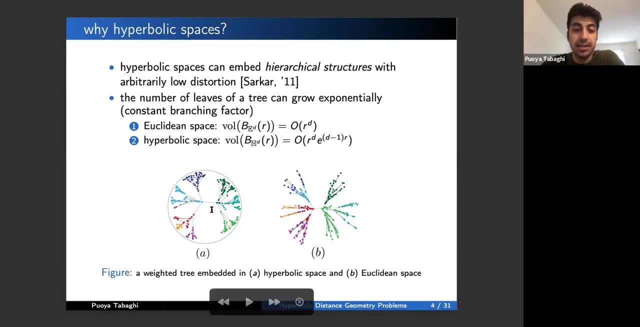 put them in B in Euclidean space and in A in hyperbolic space. So the goal of the embedding is to represent these pairwise distances that are defined on the tree. And then I went about doing K-means clustering on both of these, And these are the clusters I get Here. 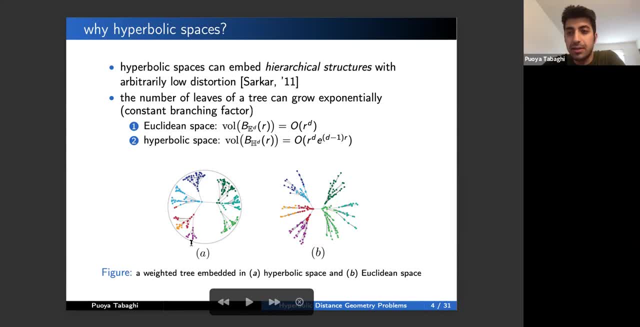 this is a Poincaretis. This is a hyperbolic space. I will get to talk about it later, But visually we will have more meaningful clusters in hyperbolic space And this is due to the fact that our embedding was more faithful, represented those pairwise distances on a tree better. So because 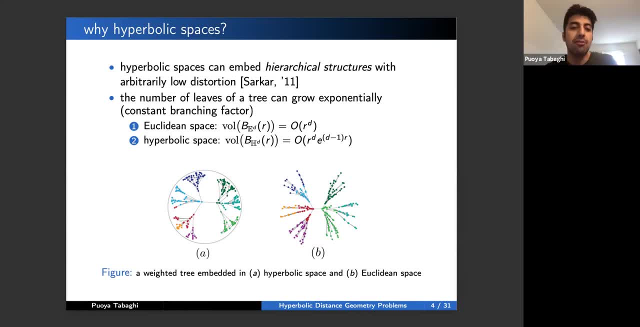 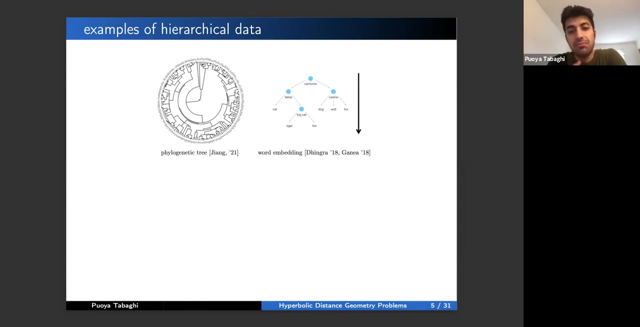 we have better embedding, then we can have clusters that are meaningful, and that is actually what we want to do. So um, There are other examples of hierarchical data, For instance. I talked about word embedding applications. You can also have phylogenetic tree where you have, let's say, a set of 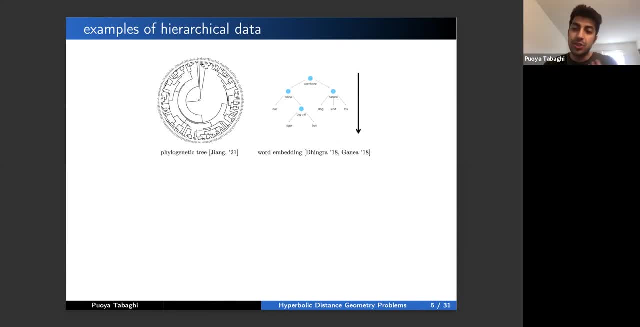 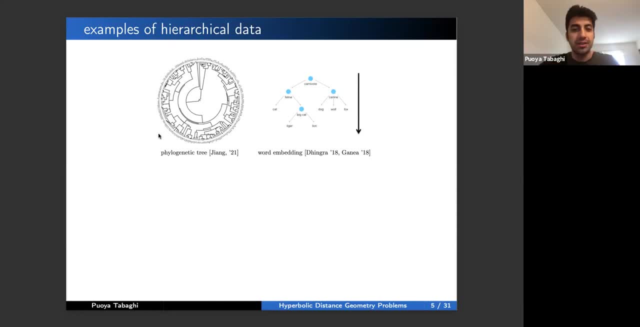 On the other hand, if you, if you want to embed just one tree model and do like, like, do like subsequent, like tasks, like, Like, placing a new node on the tree or placing a new marker organism in the onda tree, So then you need vector representation and embedding, but it's up to everybody to determine which work done in line nodes would work in that lecture, isjonary, and this is what you'll get from out of everyone's eye. You may use some image presenter tools, lineage model or some. 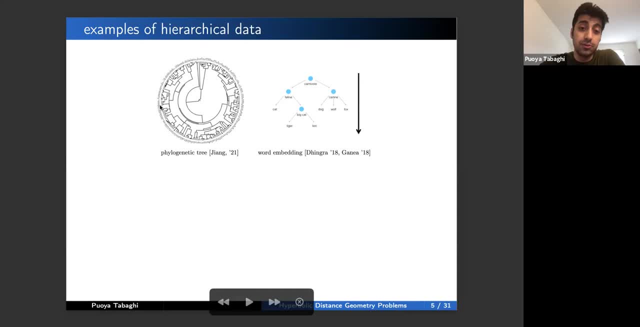 So we're arguing that if you do that in hyperbolic space, you will get better results because you can have a better embedding. Another application could be again in biology, where this is a NatureCom paper in 2020, when they showed, they reasoned that cell developmental processes can be thought as moving trajectories along trees. 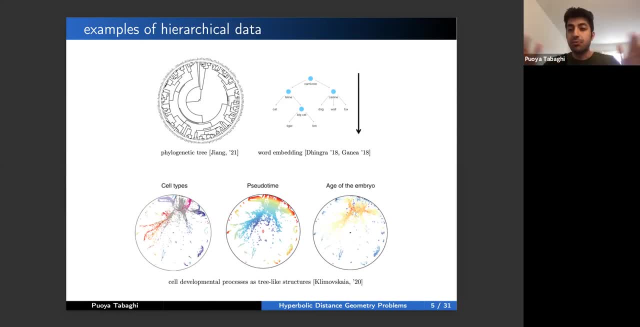 basically immature cells getting branched out and develop into more mature and specialized cells, And this can be represented via a tree, And so they defined similarities between these cells And they went about embedding these similarities in hyperbolic space, And the goal is to do a whole lot of tasks such as visualization, lineage detection, pseudotime inference and so on and so forth. 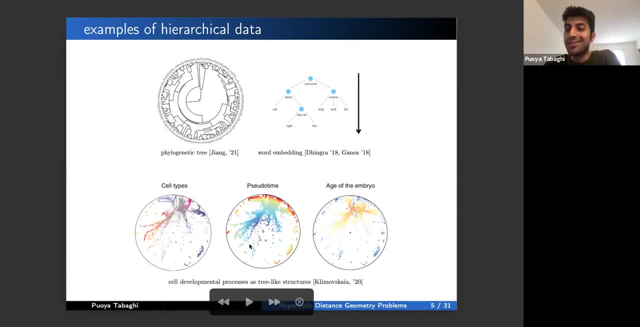 And so this is an example of that embedding, And they argue that doing these in hyperbolic space would give you a better performance compared to the Euclidean space. And, by the way, this is just two-dimensional hyperbolic space. Okay, so for all these reasons, I'm considering solving a distance geometry problem in hyperbolic space. 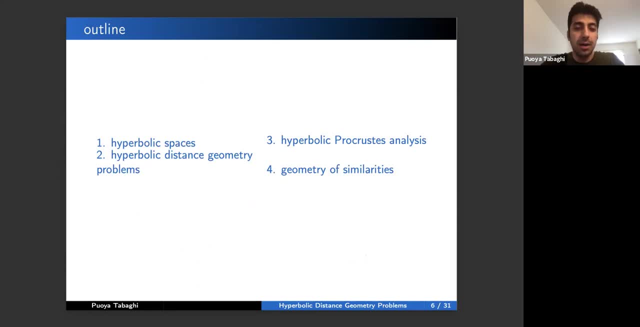 So here's the outline of the talk. I'm going to talk about what are hyperbolic spaces and what is a distance geometry problem, And then I will talk about procrosses analysis in hyperbolic Hyperbolic space, which is, you know, quite common in. if you're trying to solve a DGP in Euclidean space, you want to be able to align point sets. 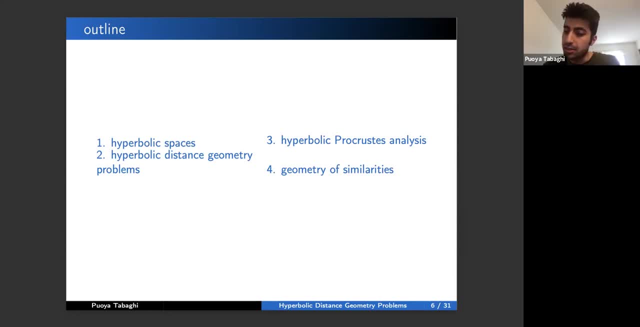 And then, finally, I will end the talk by asking the kind of a fundamental question and kind of abandoning this, you know, tree-like structure, talking about just similarities in general, And if they entail any geometrical information, Or if you can derive some geometrical information from similarities or not. 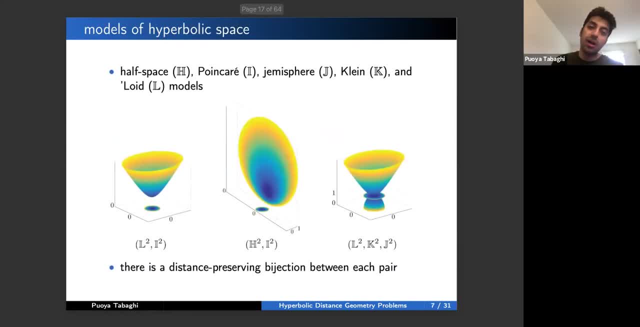 And the answer is yes. Okay, so hyperbolic spaces. There are five different models of hyperbolic space and here are all of them: Half space, Poincaré, Hemisphere, Klein and Lloyd, And in most machine learning there are five models of hyperbolic space. 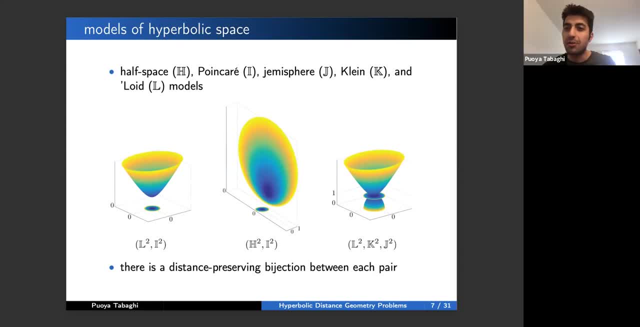 papers that utilize hyperbolic spaces in their work. they consider Lloyd and Poincare model. just because Poincare model is this disc right here and it can be used to visualize like hyperbolic points, which I just did like two seconds ago. 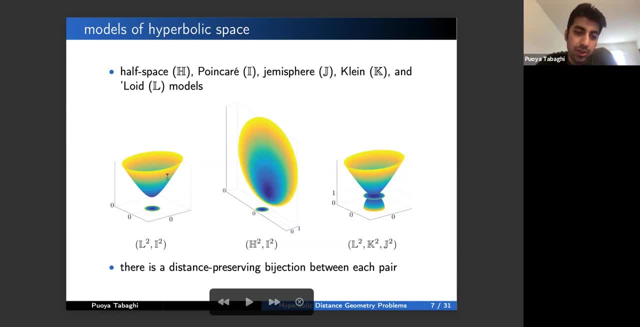 but Lloyd model, which is this hyperbolic, is, in my opinion, is pretty good for optimization purposes. But as far as distance geometry is concerned, all of these models are equivalent because there is a distance preserving bijection between all of these spaces. So if you can embed your points in one of them, 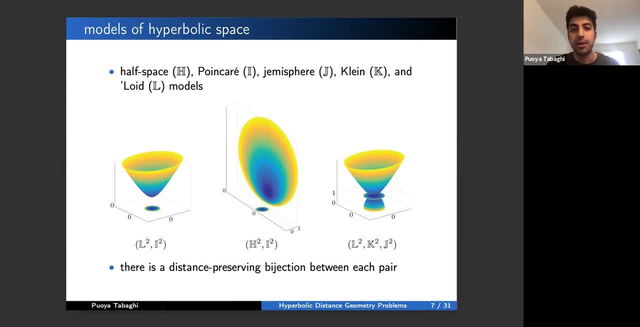 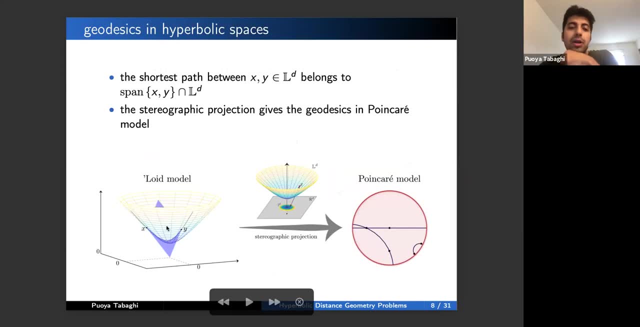 you can just transfer them to some other space and visualize it there. Okay, so this is a Lloyd model and we wanna know what is the shortest path between two points in the Lloyd model And like, geometrically it's quite easy. You can have X and Y and you take the span of X and Y. 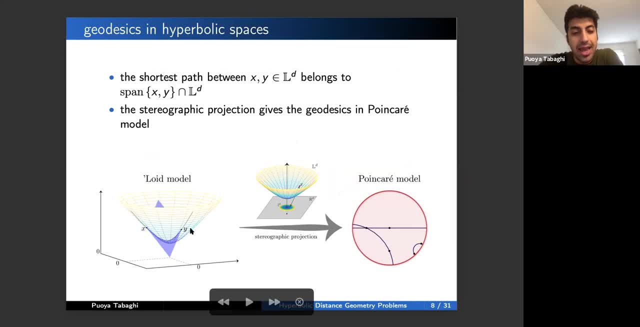 which is a 2D subspace, And then you take that intersection with the hyperbolic sheet And then this line. this line would be the shortest path line, AKA geodesic, And you can use this bijection that I just mentioned. 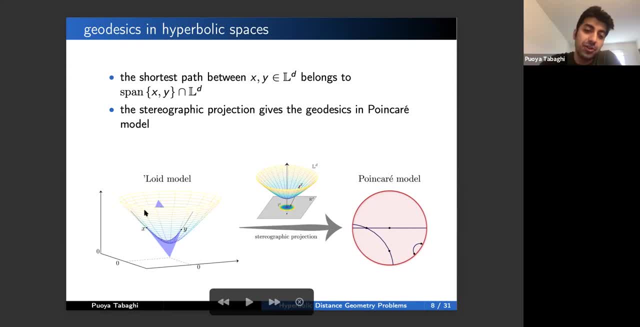 stereographic projection to basically visualize this geodesic endpoint frame model as well. So, as you can see, the lines don't look as straight, but they are shortest path lines between these points And the closer these points are to the boundary, the more curved they're gonna look. 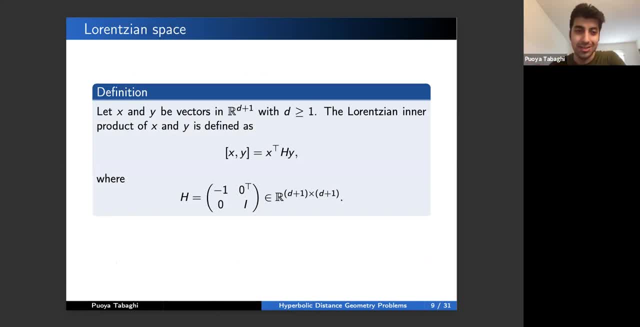 Okay. so before formalizing what Lloyd model is, we have to know one very important and simple definition, And that is Lorenzian inner product. Lorenzian inner product between two vectors in Rd plus one is defined like this: X, transpose, Hy. 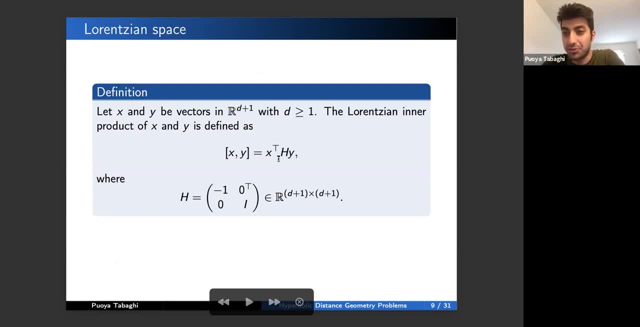 Okay, H is an indefinite matrix, So it's a diagonal matrix. Its first element is negative one, All the other elements are one, And so this is an indefinite inner product, but from here on I'm just gonna call it inner product. 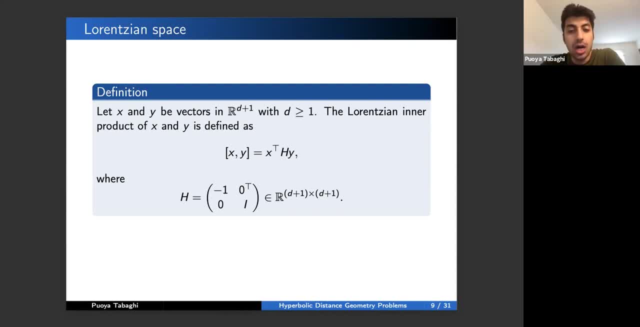 because it's gonna show up quite a bit of time. It is indefinite because if you take X and multiply by X, it can be negative right, Because H is indefinite. So with this inner product, a special inner product you can define like familiar notions. 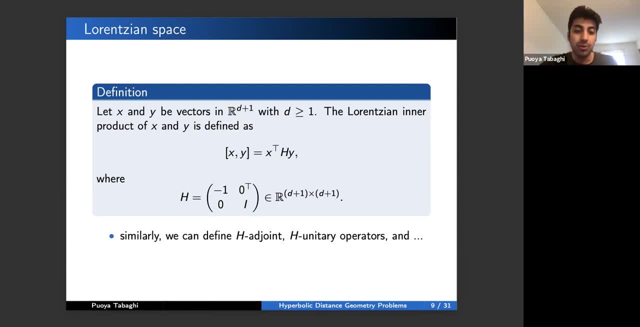 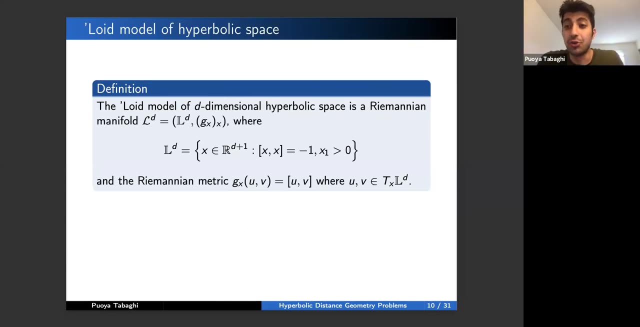 like adjoint or unitary operators, but we're gonna put an H before each one of them to make sure that we know what we're talking about. Okay, so this is the definition of Lorentzian inner product. Now we get to the definition of just the Lloyd model. 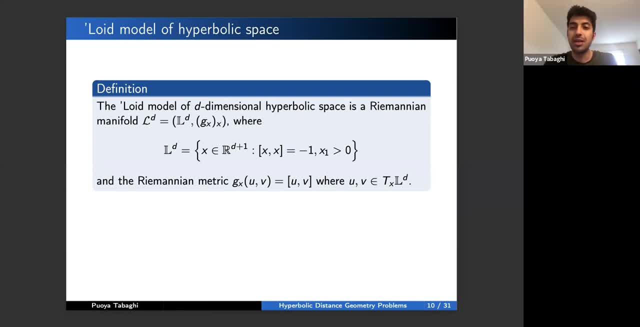 Lloyd model is a D-dimensional manifold. It's domain is a subset of RD plus one, but those points whose inner product, with themself, is negative one. Again, this is a Lorentzian inner product And the first element must be positive. 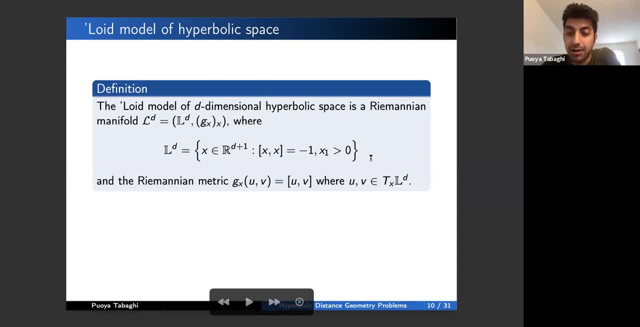 So the domain is fully characterized by this Lorentzian inner product And the Riemannian metric. there is constant for any base point that you choose And again, is defined by the inner product between these tangent spaces, tangent vectors. So basically, Riemannian metric for anybody. 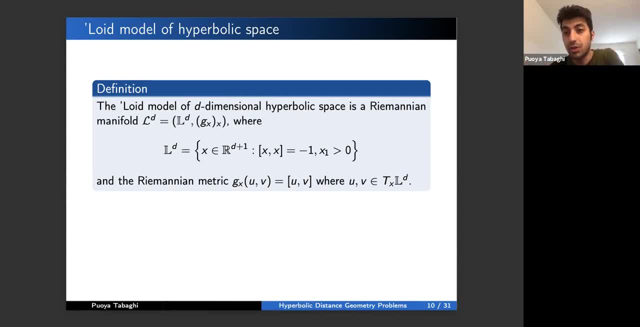 who is not familiar, is a generalization of inner product for manifolds. Okay, so the manifold is fully characterized by this Lorentzian inner product. Also the distances, the close form distances. also the distances, the closed form distances. 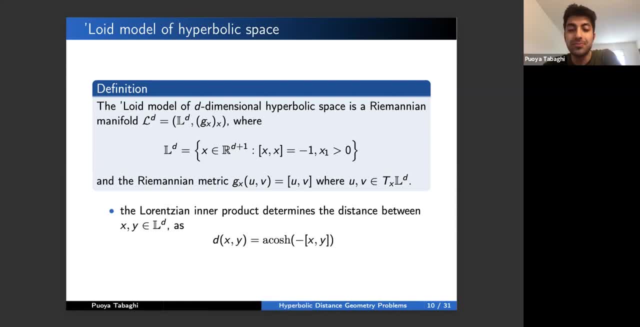 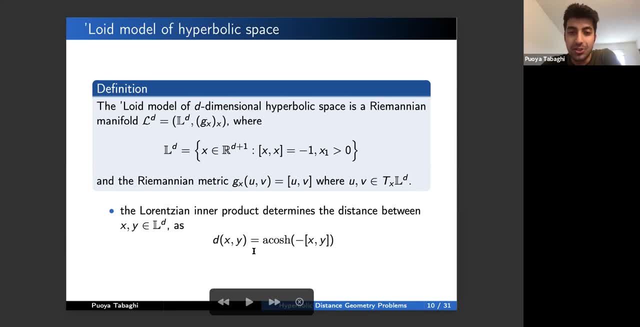 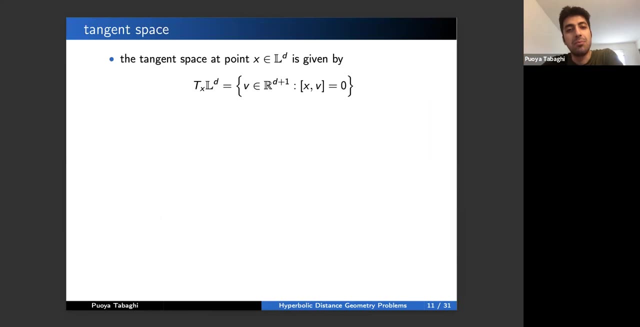 and y will give you the distance between x and y. So it seems very crucial that we should really get to know Lorentzian inner product before trying to solve anything in hyperbolic spaces. Okay, I talked about tangent spaces, but so this is kind of a tangential slide. 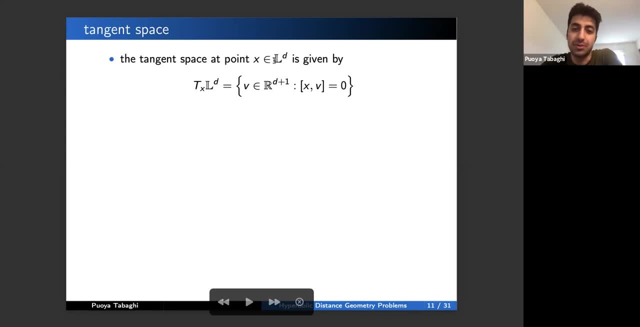 So I'm going to just tell you what it is. The tangent space at point x of the Lloyd model is basically all the points whose inner product with x is zero. Again, this is characterized by this Lorentzian inner product of x. 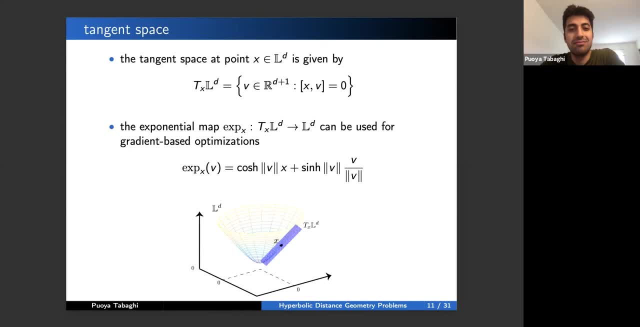 It's characterized by Lorentzian inner product, And so usually so I don't do that. but if anybody want to do a kind of implement a learning method that is gradient based, So then you need to know how to move on this manifold, And the way you move is you move in the tangent space and then 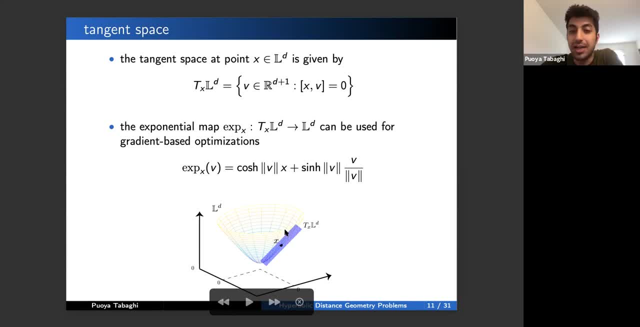 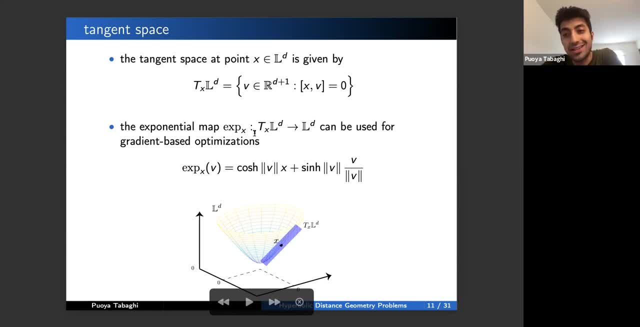 project, a vector in the tangent space at x, to the Lloyd model, And this is the expression for it, And all of these norms and everything again is with respect to that Lorentzian inner product. So Lloyd model, in a nutshell, is fully characterized by Lorentzian inner products. Okay, 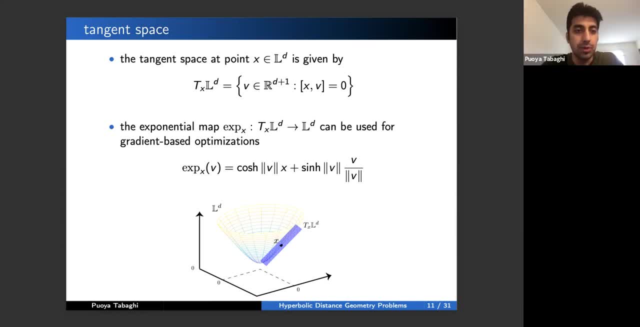 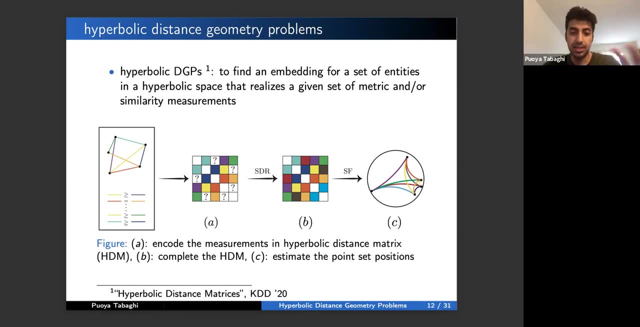 So now that we identify what Lloyd model is, let's formalize what distance geometry problems are. Okay, So this slide is basically as the pipeline of solving any distance geometry problems in hyperbolic spaces with if, if, if. we are trying. 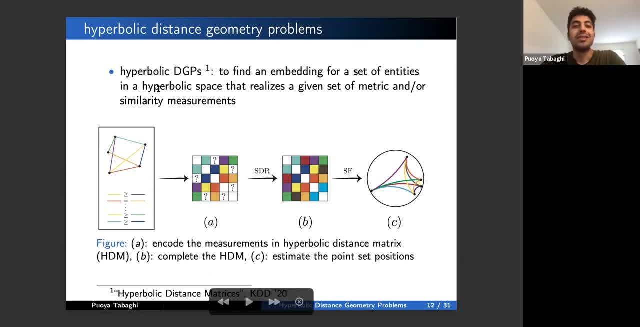 to solve it with semi-definitive relaxation. So okay, Let me. let me explain what hyperbolic DGPs are. We want to find an embedding for a set of entities that realizes a given set of distances, or similarity measurements, or and similarity measurements. 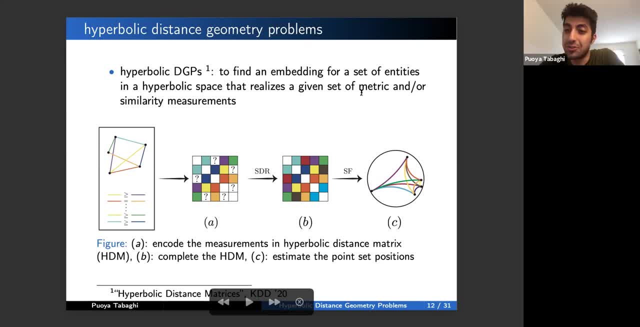 So distances are what I call metric measurements and similarities are what I call non-metric measurements. So I I kind of represent these kinds of measurements in this box. Metric measurements is where we know the distances between pairs of points, and non-metric measurements. 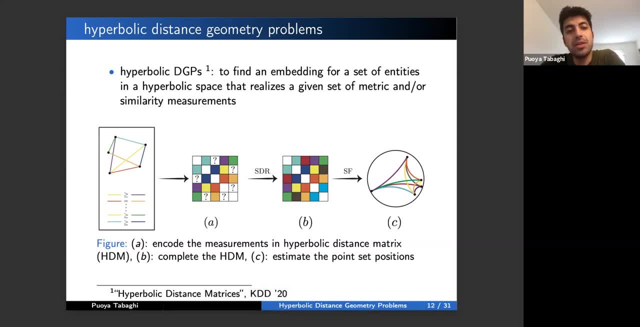 between pairs of points and non-metric measurements. Okay, So this is where we know the distances between pairs of points and non-metric measurements, Right, Okay? So what are some of these? And then, of course, have alpha, and alpha is going to be lg, which are the 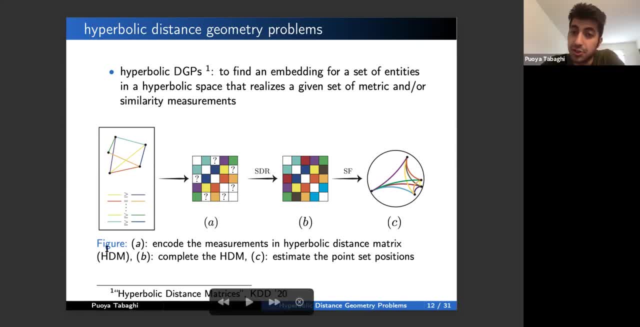 gamma and otrake points that we're looking at here, Right, And so these are the set of points that we're looking for. distances, different pairwise distances. So we have these measurements and I'm going to encode them or tabulate them in a matrix n by n, matrix that basically represent all of the pairwise. 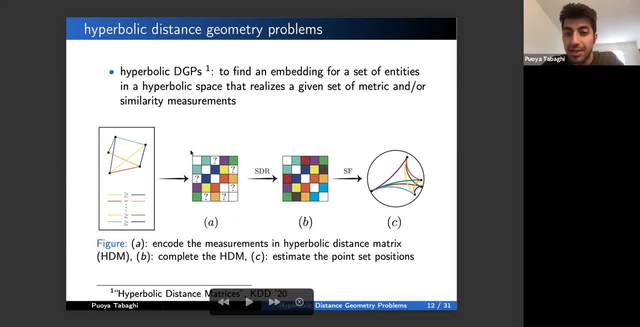 distances between these entities. So this is a distance matrix. So, as you can see, we might not have all of the distances, but we might have some of them and they can be noisy, And I will show that with a semi-definite relaxation, we can denoise this matrix and estimate the missing. 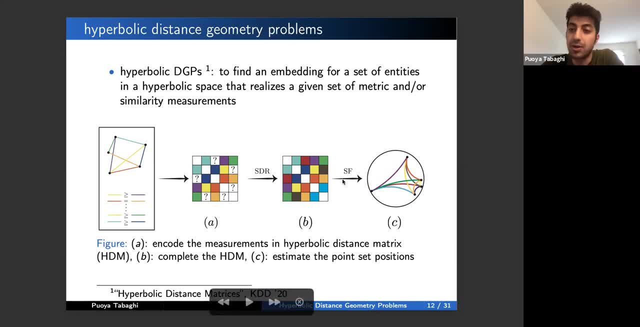 measurements, And once we have all of the pairwise distances, then we can do a simple spectral factorization of this matrix to estimate the point positions here in hyperbolic space. Okay, So this is the whole pipeline, So I'm going to talk about distance matrices. 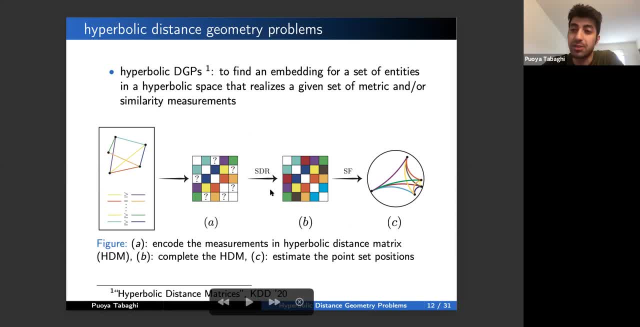 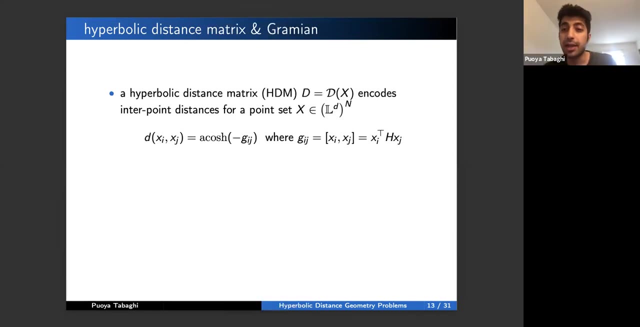 and what semi-definite relaxation means or semi-definite characterization of these distance matrices are. And then I'm going to finish with the spectral factorization. So okay, So a hyperbolic distance matrix encodes all the pairwise distances for a set of points in the Lloyd model. 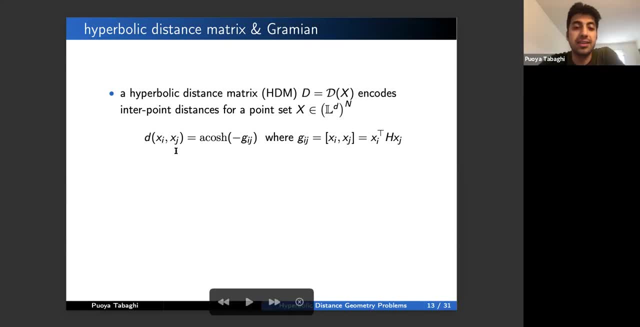 Okay, So distance between X and I and XJ, as we mentioned, is inverse hyperbolic cosine of their minus inner product, And the inner product is defined like this right. So this is a Lorentzian inner product And HDM is basically a collection of all of these pairwise distances. 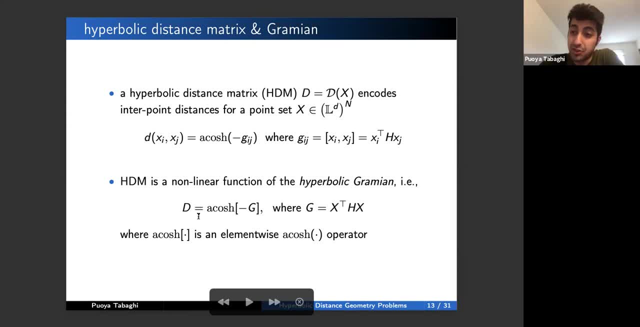 which we are going to put it in the matrix D, And we could, we put the intersection of all of these pairwise distances in a matrix called G, which is hyperbolic, Gramian because it encodes all the pairwise inner products, And it is hyperbolic because the points are hyperbolic. 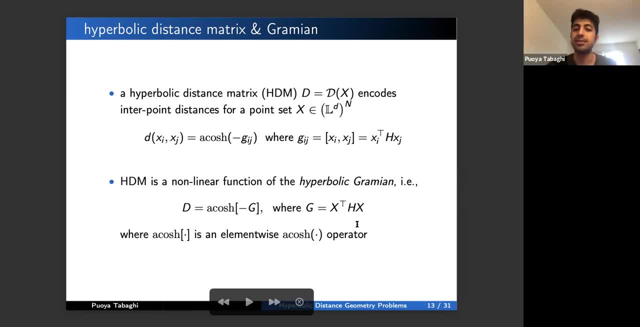 And this G can be written as X transpose HX, So again we have this H in the middle. So this G matrix is not a semi-definite variable And we want to solve this problem with semi-definite relaxation, So by lifting the parameters from X domain to G domain and finding a semi-definite. 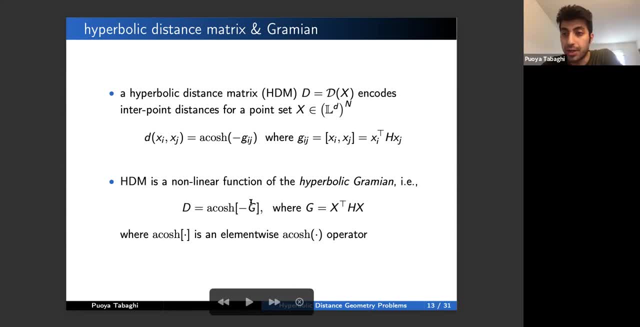 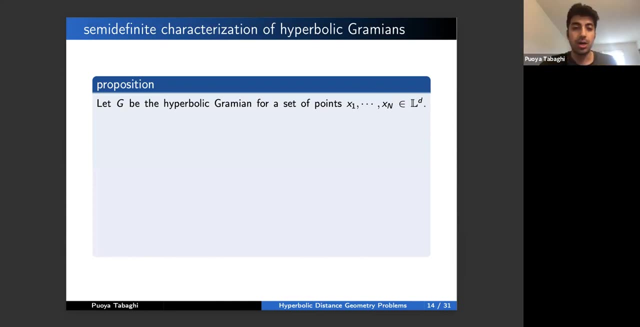 characterization for this G. we're hoping that we get to the place that we want. So in the next slide I'm going to talk about how to represent this G in terms of positive semi-definite variables. Okay, So this proposition basically formalizes our claim. Let G be a hyperbolic Gramian for a set of points and points. 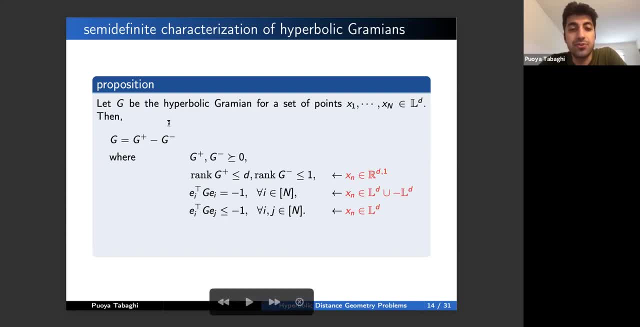 So then we can write G in terms of subtraction of two positive semi-definite matrices. Okay, So G is not a semi-definite matrix, right? And there is going to be this rank constraint for G plus and G minus, And this is to ensure. 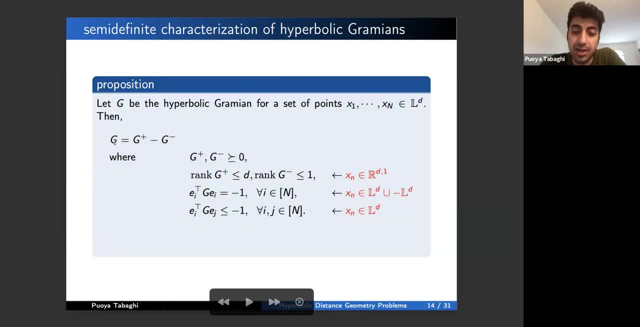 that this G here encodes all the Lorentzian inner products. this rank constraint And all the diagonal elements of G must be equal to negative one, And this is to ensure that the inner product of every point wood itself should be negative one by definition. 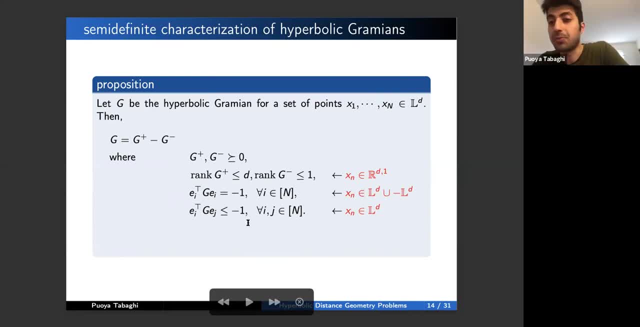 And then all the off-diagonal elements should be less than negative one, And this is that technical thing to ensure basically all the points belong to one sheet of hyperboloid, because you can have two sheets of hyperboloid, Anyway. so this is a semi-definite characterization of hyperbolic Gramian. 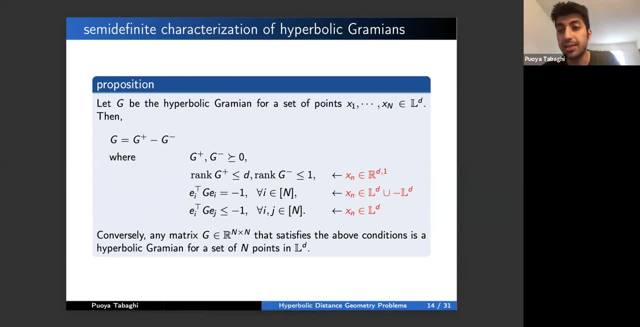 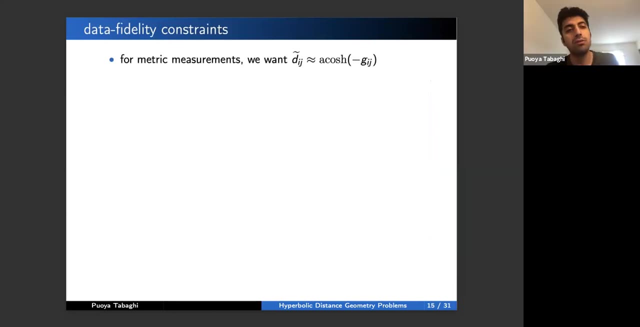 By the way, we have the converse as well. so any matrix that satisfy these constraints is a hyperbolic Gramian, So a proper hyperbolic Gramian for some endpoints in d-dimensional space. Okay, so now we want to solve DGP in hyperbolic space. So for metric measurements. 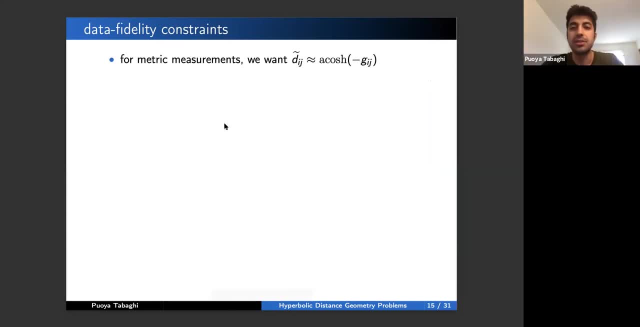 where we have the noisy pairwise distances. we want this condition to hold. We want Dij, which is the noisy measured distance, To be approximately what we get after embedding the points right. But this is a non-linear function of our parameter Gij. so what I'm going to do? I'm going to take hyperbolic cosine from each side. 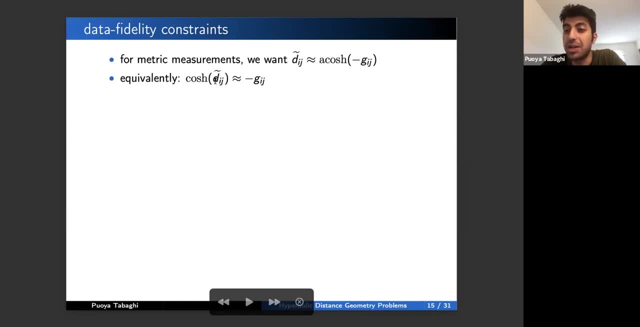 and I'm going to say, okay, we want hyperbolic cosine of our measurements to best represent this parameter. And if I do that for all ij's, that I have the measurements for metric measurements, then I can have something like this Hyperbolic cosine of all of the measured distances. 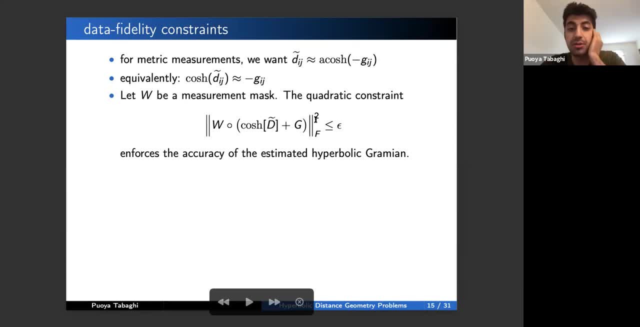 should best represent minus G. so plus G here and I will measure it at the, at the indices that I have the measurement for right And I want this error to be less than epsilon, That's. that's that's data fidelity constraint that I'm going to have for my semi-definite program. 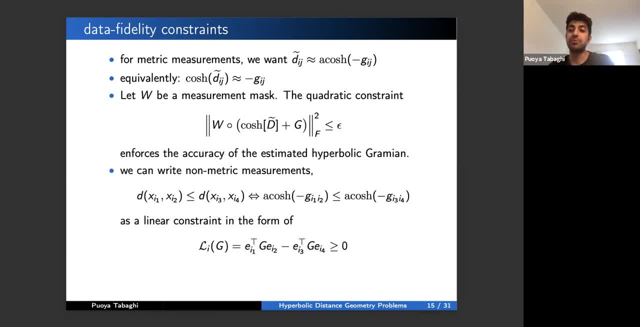 And, as I mentioned, non-metric measurements are basically distance comparisons. so we have these constraints, We want. we want some distances to be less than some distance, some other distances based on the similarities that we measure. So, if we follow the definition, 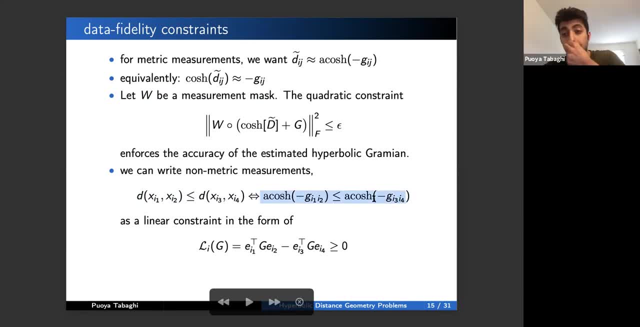 we have this and because inverse hyperbolic cosine is monotonic function, then we would have- they will have- this constraint as a linear inequality constraint on G basically. So the bottom line is linear and quadratic data fidelity constraint can impose a good embedding like constraint for metric and non-metric data. 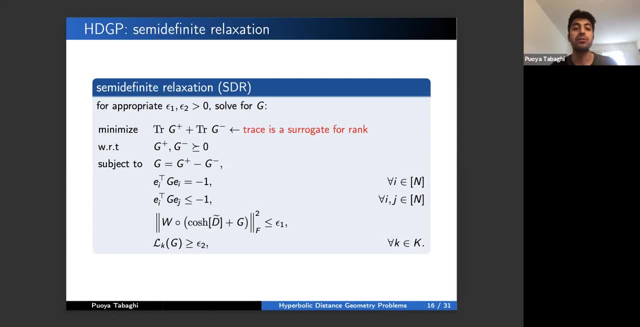 So this is our proposed semi-definite relaxation to solving this problem. So we want to minimize the rank of those two matrices. So instead we say, okay, we can't do that, so let's minimize the trace as a surrogate of these matrices With respect to them being positive, semi-definite. 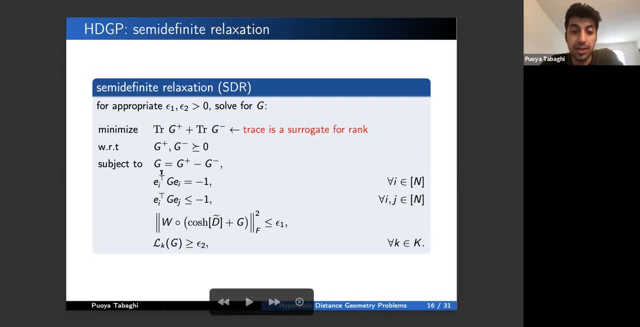 their difference should be hyperbolic Gramian. It has to satisfy the hyperbolic Gramian conditions And also during the embedding, it also has to satisfy some data fidelity constraints. You can see that this is a linear inequality constraint. It has to respect the measurements. This is a 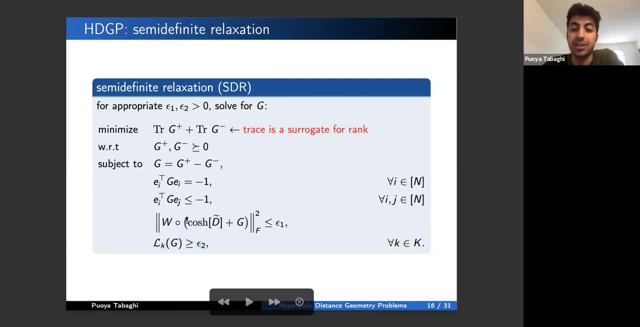 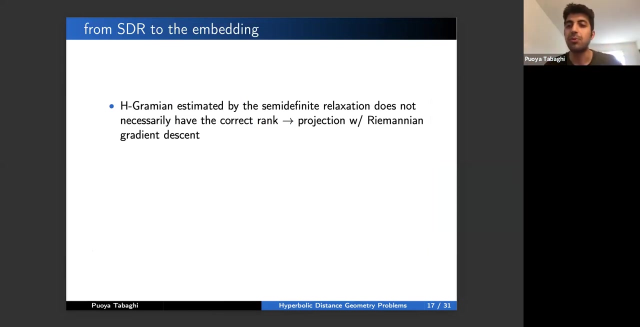 metric measurement and this is non-metric measurements. So this is a linear inequality constraint and this is quadratic constraint, And these are linear. so this problem can be solved relatively easy with available SDR packages. Okay, so after you solve these for G plus and G minus and you come up with your hyperbolic Gramian. 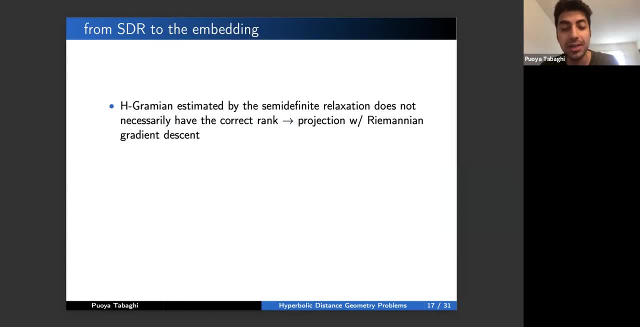 almost surely the rank of this matrix is not going to be correct because we relaxed the rank constraint. So we have to do some sort of projection and subsequent Riemannian gradient descent to correct the rank. So I'm not going to get into detail of that. but let's assume that 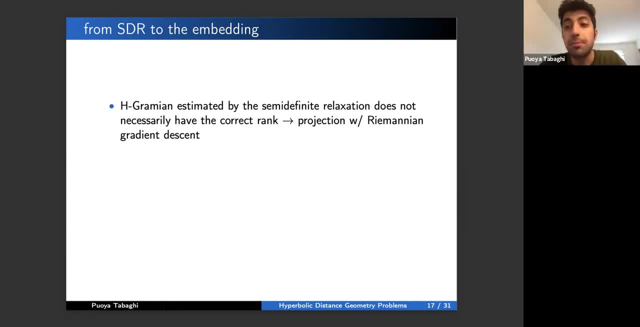 we've done that, And now we're going to solve for the hyperbolic Gramian. So let's do that. So let's we have a hyperbolic Gramian of the correct rank. how do we go about estimating these point positions? 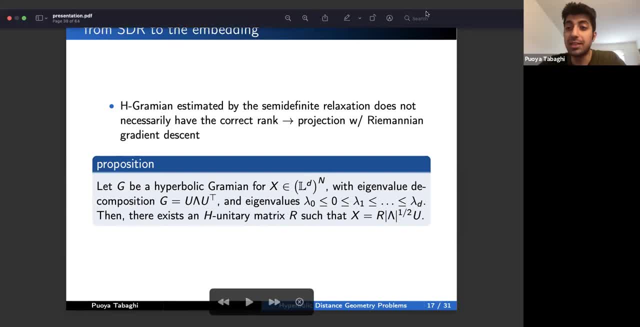 at the end. So it's really easy. a simple eigenvalue decomposition on the G would give you eigenvalues that are positive and negative, So you take absolute value of that, the square root of them, multiply by the eigenvectors and you have your point sets. 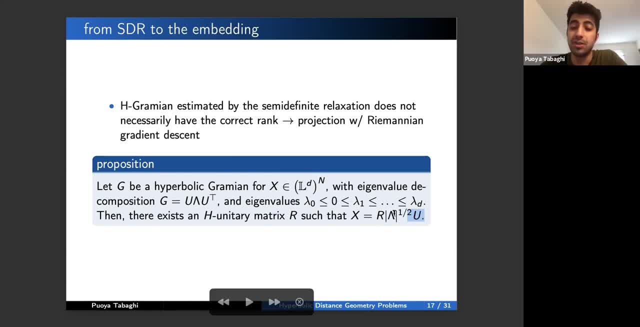 But here R is not your average unitary matrix that you have for Euclidean spaces. This is, as you guessed. this is an H unitary matrix because of the Lorentzian inner product business that we talked about. So there's this ambiguity. 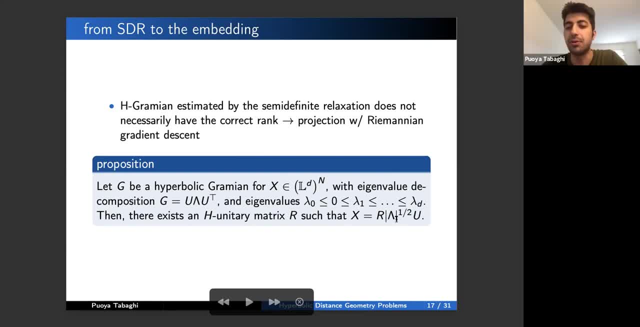 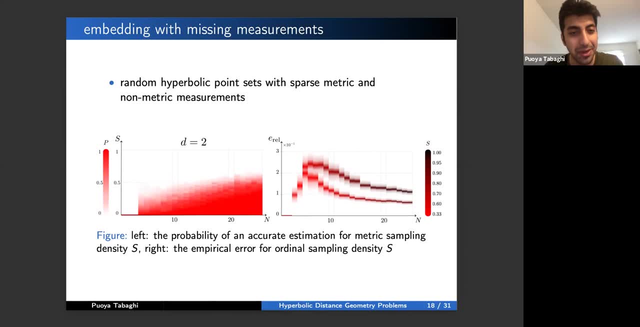 We don't know the exact location of X, but we know it up to an isometry. Okay, So here we conduct an experiment. It's very like, simple: We generate random hyperbolic point sets and we measure their inner, their distances. 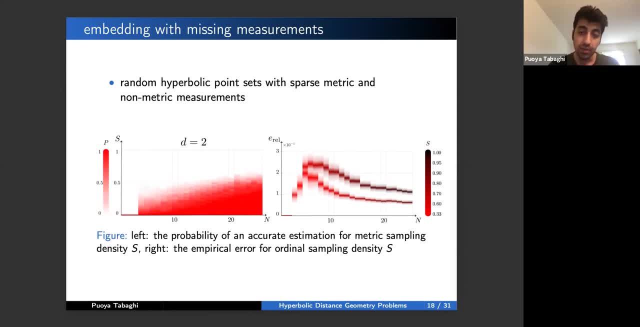 and we just deselect some of them as far as if item, And now we have a distance matrix with missing measurements and we run our semi-definitive våraósqueto matrix, Okay, to estimate the missing measurements And we're gonna report the maximum sparsity level. 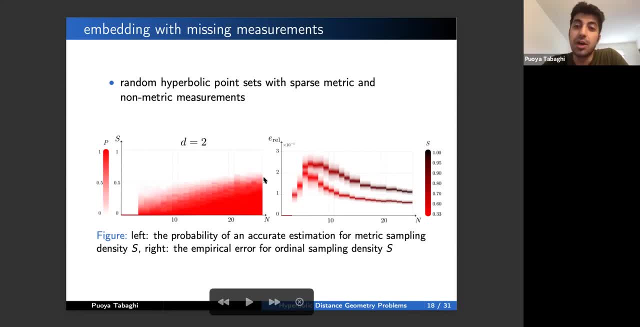 that this semi-definite relaxation can take while giving us a good reconstruction- And this basically shows the maximum sparsity level- grows with the number of points that you generate, And so this is kind of similar to Euclidean spaces as well. So the more points you have, 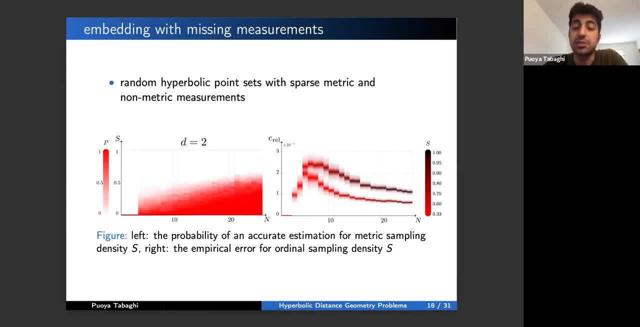 the more, the sparser your distance measurements can be, And we repeat the experiment with non-metric measurements. Again, we generate random points. We can compute their distances, but we totally ignore distances and we just retain distance relationships, Like you know. 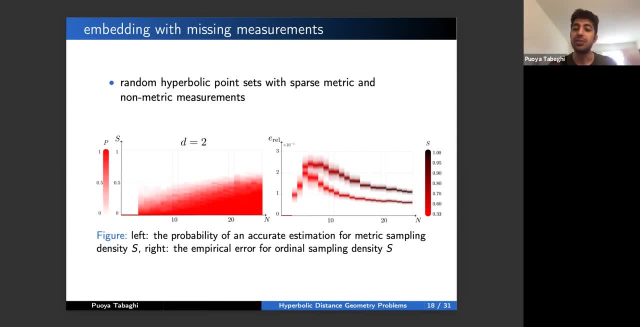 we can't compute the distance relationships because we can't compute the non-metric measurements, And we subsample those inequalities or non-metric measurements and we embed those basically inequalities, basically inequality measurements or non-metric measurements. And here's the relative error. 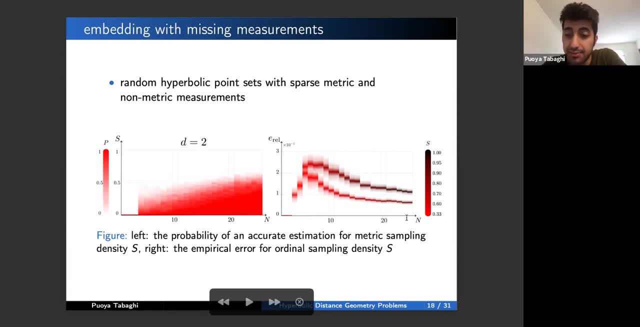 embedding error that we get as a function of, like the number of points, It goes down. Also, we get to have- this is a sparsity level. We get to have a sparser and a sparser measurements, for the more we have, the more number of points we have right. 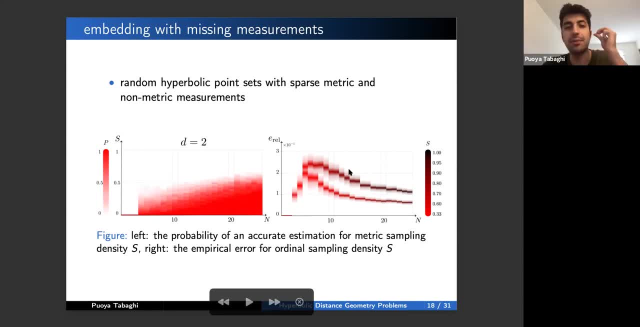 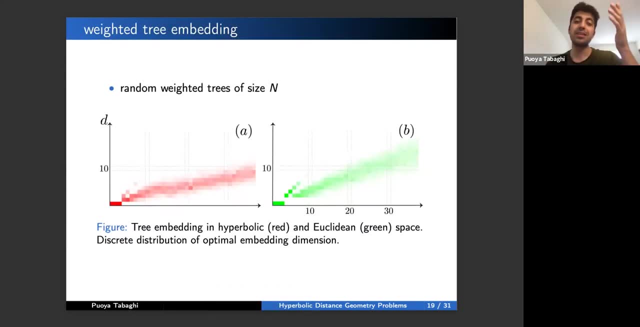 So it does a good job for metric and non-metric measurements, for just purely hyperbolic point sets. So we're going to repeat the experiment with like weighted trees. Now we generate random weighted trees with random weights and we embed them. We embed them in hyperbolic and Euclidean spaces. 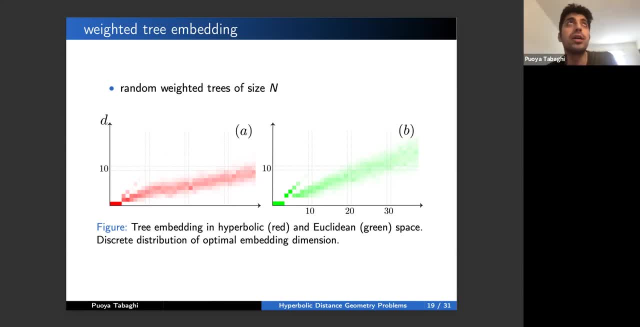 But this time we're going to change the embedding dimension and we're going to find the best, or like the minimum embedding dimension, that the embedded points are that satisfy a certain accuracy level, Like they should. pairwise distances should accurately represent those, those that are from the tree, and so for each realization, for each random tree we have, 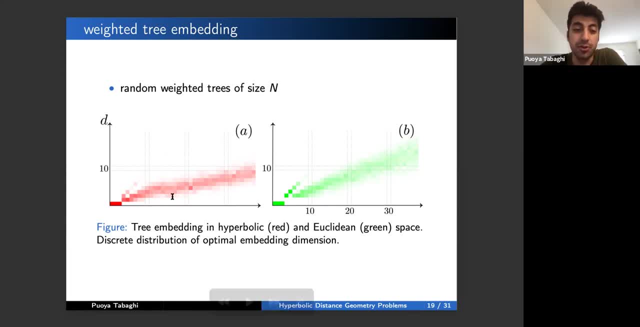 a specific optimal embedding dimension for hyperbolic and euclidean. and here you see, the y-axis is embedding dimension and this is basically the distribution of embedding dimension. red is for hyperbolic point sets, sorry for hyperbolic embedding, green is for euclidean embedding and this x-axis should be the number of points in the tree. so the optimal embedding 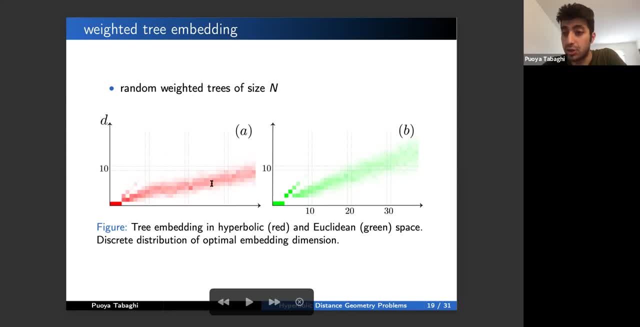 dimension for euclidean spaces is growing faster than uh hyperbolic spaces, and that again stands for the fact that if you, if you're dealing with weighted trees or any tree like a structure, you're better off embedding them in hyperbolic spaces, at least in dimension, and 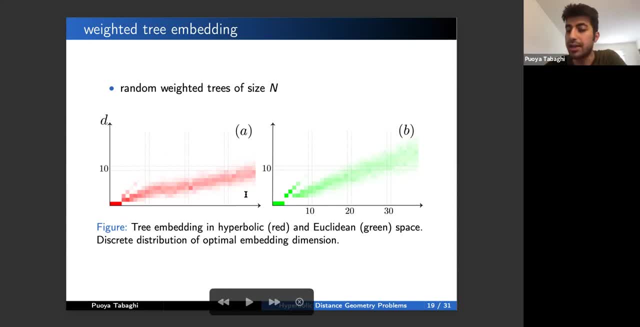 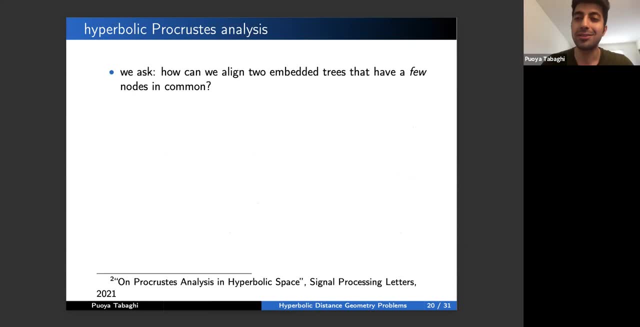 and and and and, in some ways in accuracy as well, Okay, Okay, so this was solving hyperbolic distance geometry problems. Now, as many of you are aware, in solving DGPs, usually you have ambiguity in the exact location of the point sets. 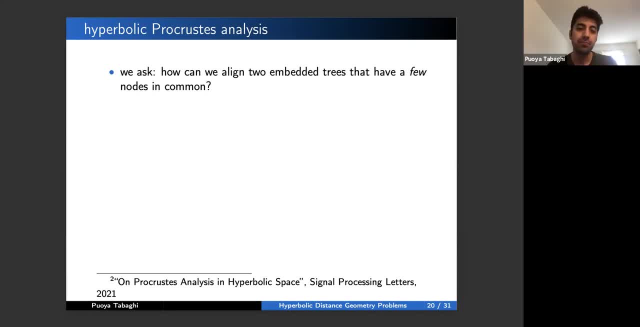 You need some anchors to find them. So, and that's the problem, That's what progressive analysis is trying to solve, right? So here we say: how can we ask the exact same question while we have like kind of this tree language? 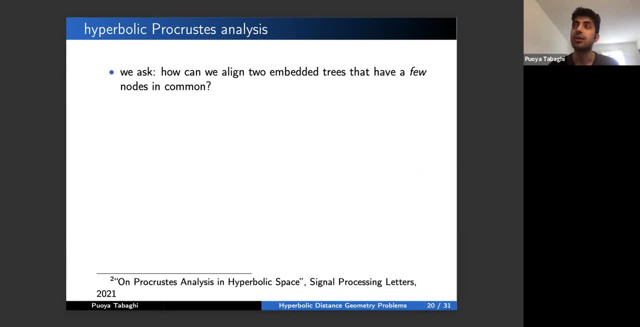 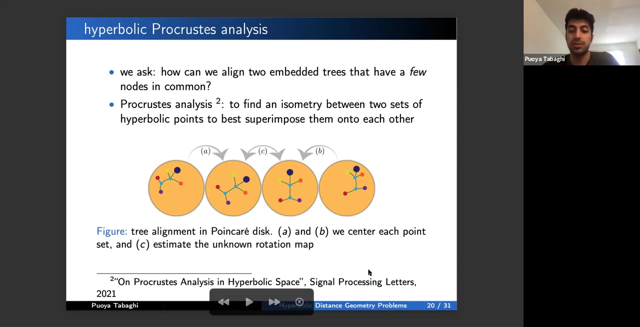 How can we align to embedded trees that have few nodes in common, Like now? aligning means like finding an isometry or distance preserving map that best basically superimposes these two structures together. So the answer is progressive analysis, And we just had a paper that was accepted. 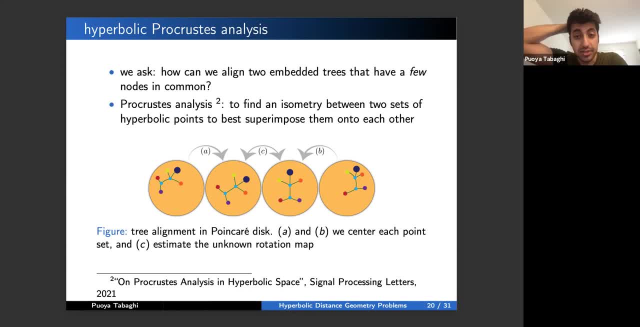 in signal processing letters on it, And the idea is to find an isometry between two sets in hyperbolic space that best superimpose them together, And here's like a cute visualization for it. So we have the far right and far left point sets. 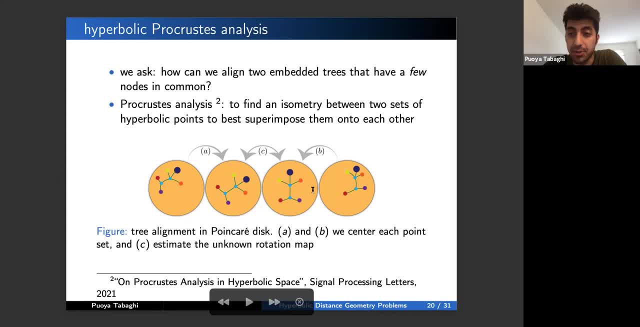 And we know that they are related through an isometry: the distance preserving map. How do we go about estimating this map? Well, it's really easy. It's quite similar to the Euclidean spaces, in which we basically center each point, each point set. 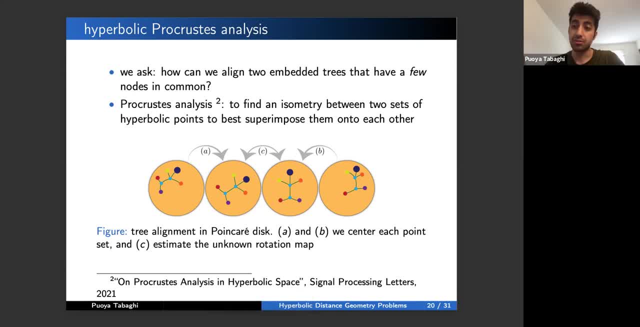 and we find the unknown rotation that basically finishes the job. And this is exactly the case for hyperbolic spaces as well, And I'm going to talk about, like, basically, isometries in hyperbolic spaces and translation rotation, and how do we go about centering point sets. 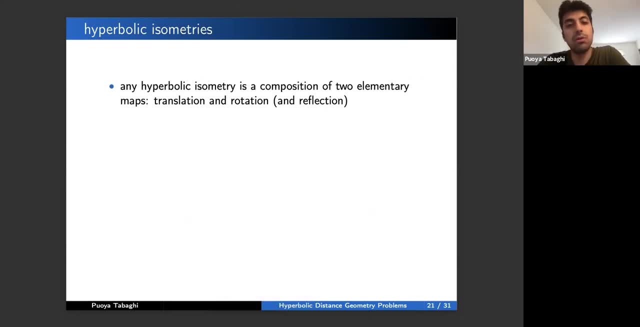 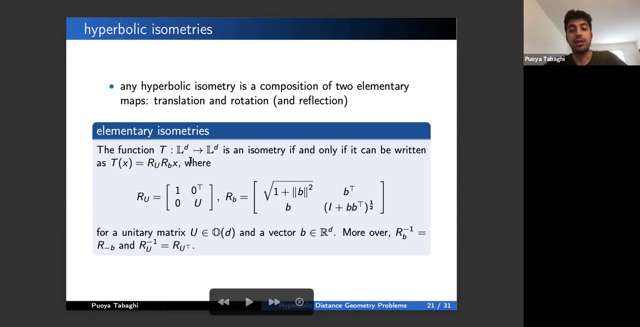 in a hyperbolic space. So our analysis is based on the fact that any isometry, hyperbolic isometry, can be decomposed into two elementary maps: translation and rotation, And they are given as follows. So if T is an isometry, 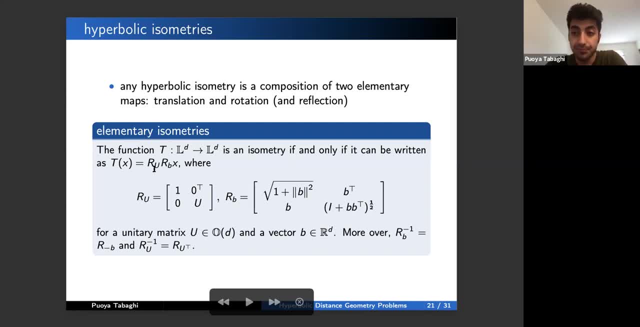 it can be written as the product of two matrices. basically, RU is the rotation, We can think about it as operator, And RB is quote, unquote, translation, And it's characterized by d-dimensional vector B here, And that B basically shows the direction. 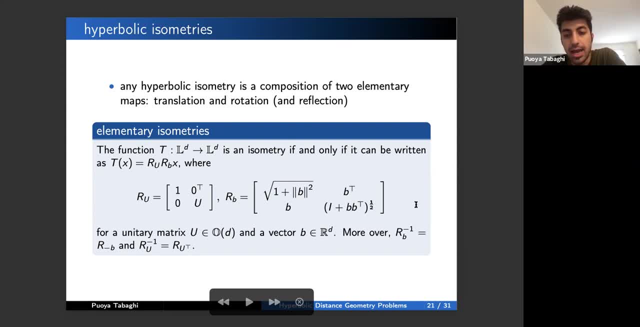 that we want to translate these points in And we call them translation and rotation And but they're like especially translation that it doesn't behave like Euclidean translation, Like it doesn't move all the points. It doesn't move all the points with the exact same. 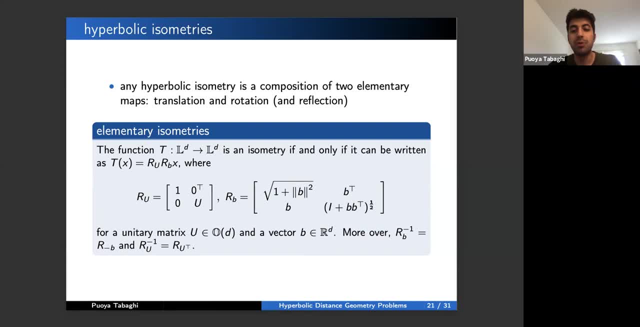 Euclidean distances, but it does have the property that we want it to have, which is RB. inverse is R minus B, which is kind of like the property that you would want to expect from a translation at least. So here I visualize these two operators: 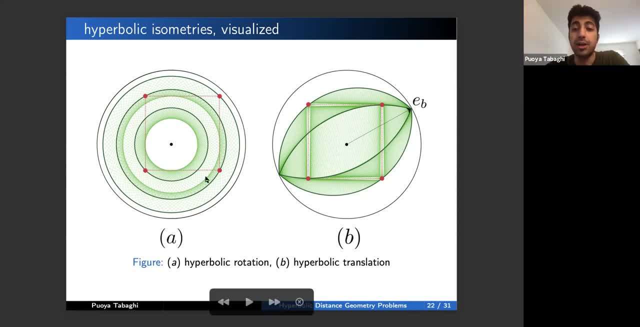 So we have four points. that's here and I'm going to- I'm going to show you how to do it And I'm going to show you how to do it. I'm going to apply consecutive rotations on these four points and I'm going to rotate them. 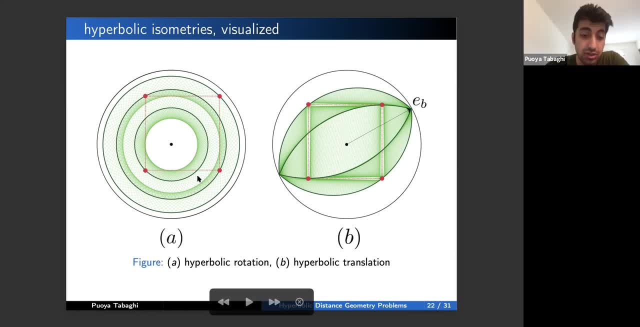 And this is the locus of the points that we get in Euclidean, in Poincaré, space, And this is just the perfect circle. So just the simple rotation means hyperbolic rotation, right, But for translation is a little bit different. 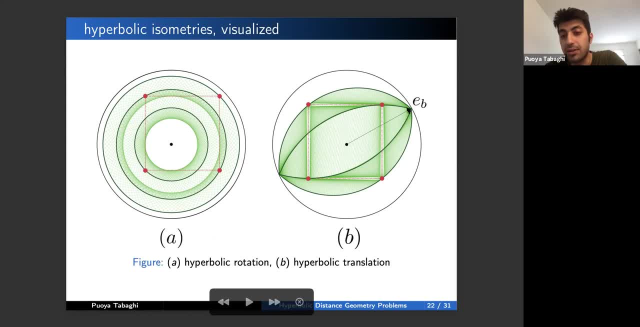 And this is, this is a direction of the translation that I'm going to define. So I'm translating all of these four points in this direction, and each time a little bit more than previous time, And this is like, basically, the locus of all of these edges. 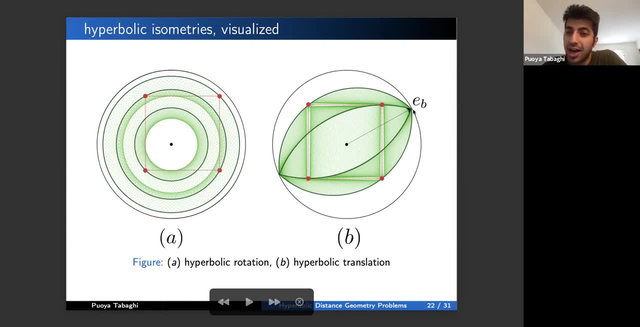 all of these vertices And, as you see, they're kind of look like they're converging to one single point. And that's okay because the distance is here near the boundary of Poincaré, this basically blow up You. they may look like they're converging to a single point. 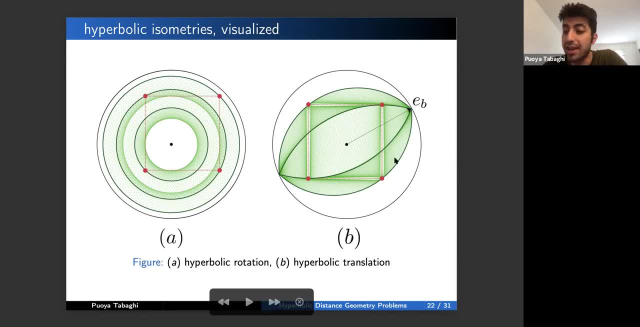 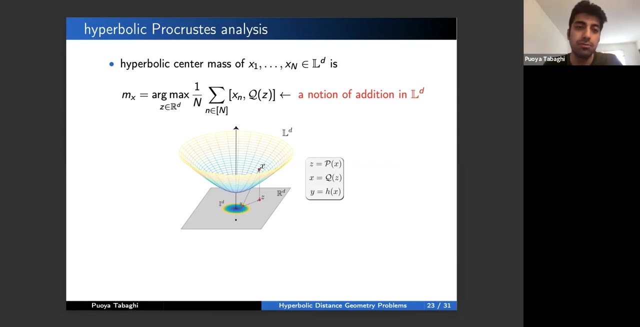 but actually all of these pairwise distances are remain intact, So so, so this is how translation works in hyperbolic space. Okay, So there are two, two problems When when it comes to solving Procrestis analysis. one is the notion of center mass in hyperbolic space. 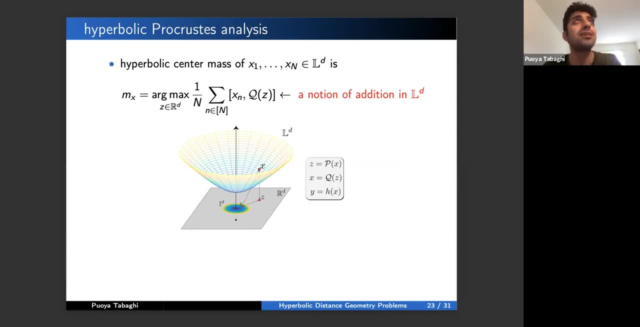 Usually in Euclidean space center, mass is the point that kind of minimizes some sort of discrepancy or variance. but here we define it kind of differently. Actually this is not my definition, you know. you can find it in the literature as the point to be maximizing some average inner product, basically. 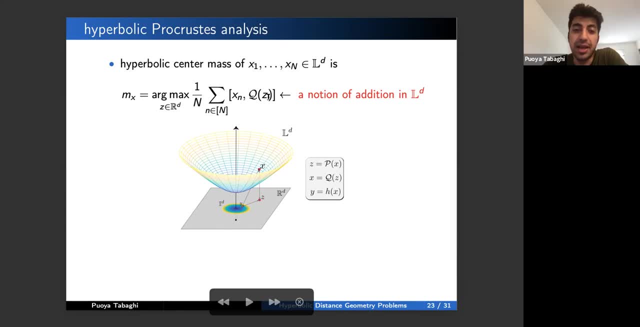 This QZ is the center mass and it maximizes some average inner product. And once we find this QZ, we map it to Z, which is in this plane, And that will be our center mass, basically. And we have the following lemma, basically, or proposition: 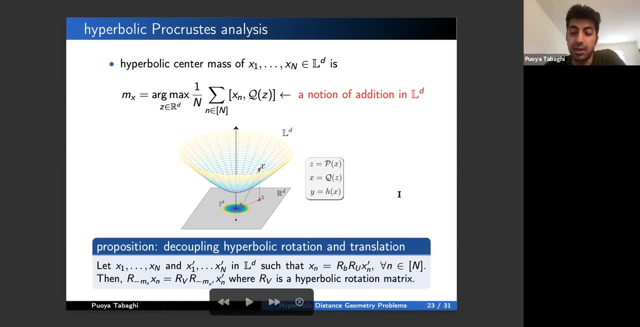 If, if you have two points sets that are related through an isometry, which is a rotation, and translation, After you center each point set, then they're only related through a rotation. So by centering we simplify the problem and we get to just basically estimate the unknown rotation. 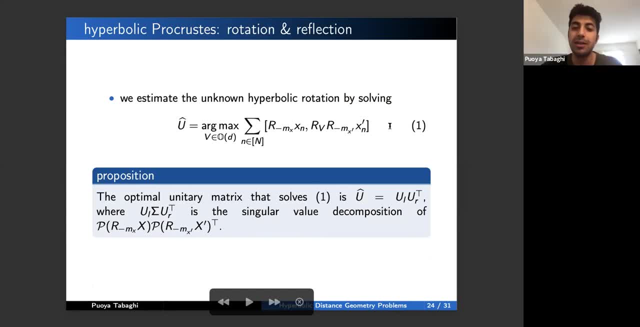 And the unknown rotation. again is really simple. We just want to maximize this average inner product, basically between centered point sets, And this can be done by a singular value decomposition very similar to orthogonal for crosses problem of this matrix, basically like centered point sets product basically. 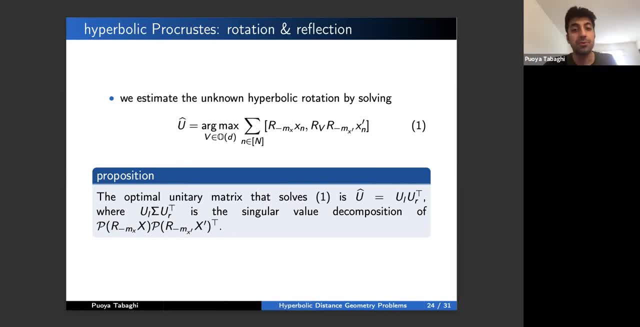 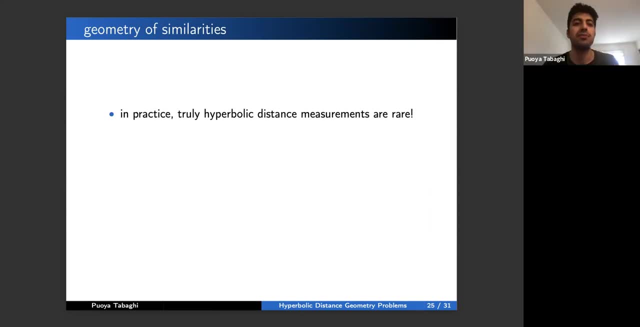 So this is, this is the gist of hyperbolic progresses. And now for the final point of my talk, and that's kind of like a fundamental problem: figuring out or trying to reveal the underlying geometry of similarities. so you know, most often than not, in practice, truly hyperbolic distance measurements are rare, unless we are, we know. 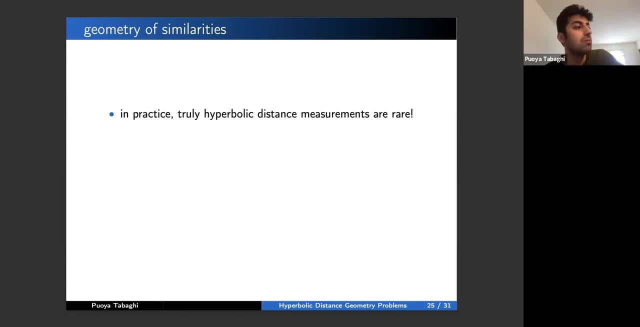 that we are dealing with trees, or yeah, or like we have some strong like assumptions or we just want to solve the problem in hyperbolic geometry, but most often we have only similarity measure. we don't even have distance measurements, we only have similarity measurements, and you know there are so many examples of similarity measurements you can. 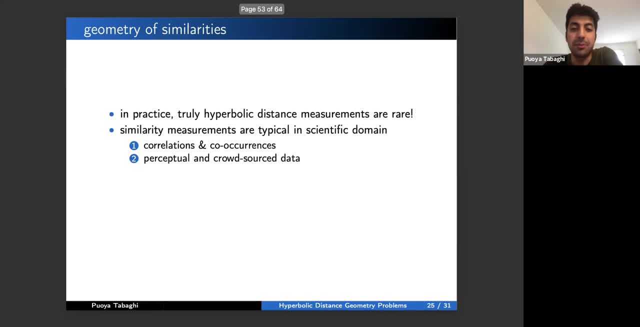 think about correlations and co-occurrences. you can think about perceptual crowdsource data. you can think about, like lots of biological data where you get to measure the activity of neurons, for instance, and compare them together. so there are so many like similarity measurements and the 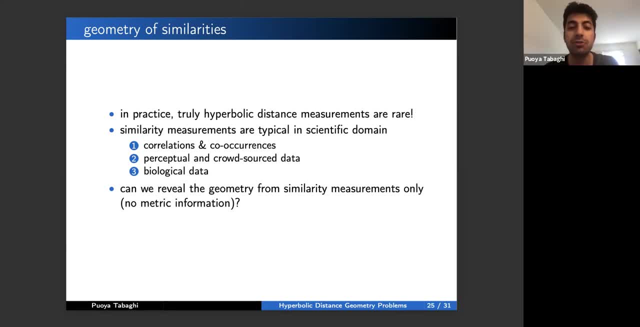 question that we're asking is: can we reveal the geometry of, like underlying geometry of these similarity measurements? uh, and we're not going to use any metric information, we don't know the pairwise distances between these entities. so this is kind of a general question and we have quite a bit of like theory about it, but i just want to convey the basic ideas that we 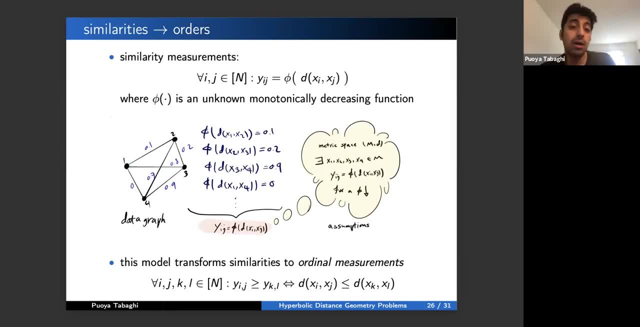 are thinking about this problem. so, um, similarity measurements, uh, we have this kind of depend on who you ask- kind of simple or very strong assumption and that is like: uh, similarity measurements yij between two points, i and j, is just the non-linear function of the distance between x i and x j. the 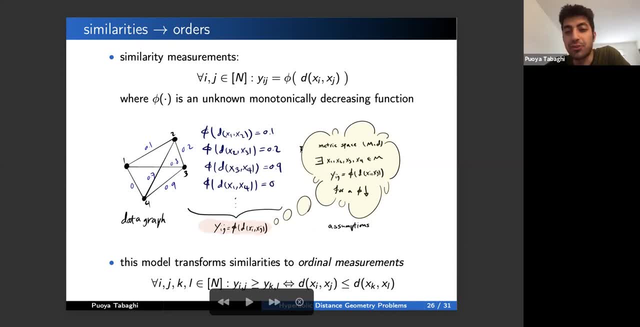 embedded points and this phi is monotonically decreasing. so if they are closer they are more similar, if they are farther away, they are less similar. um, so we are Preparing seventies and tet arbit kg, and if you talk about similarity как вещи, so like an example would be, you have a data graph and you get some measurements here and you know. 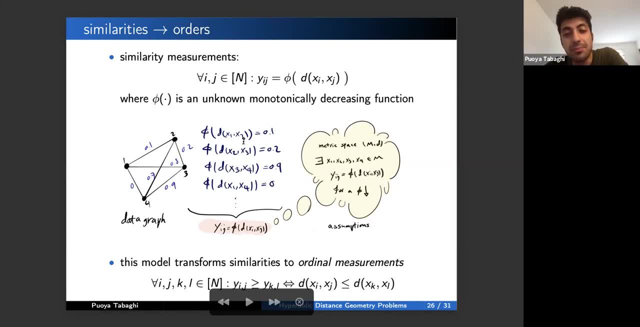 these are similarity measurements. so what this assumption basically says is that there is a metric space in which these x's reside in and there is a distance function on it, and there is again a phi- uh, unknown phi- function, such that these phi of these distances basically realize this similarity. 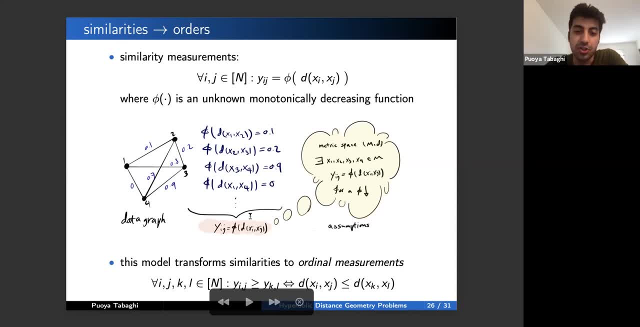 uh, measure the energy. so to this, imagine that in the input space you can look at x point. you can serafine flowing into the function these similarity measurements, right? So this is the basic assumption here And because we're assuming that this phi is monotonically decreasing function. 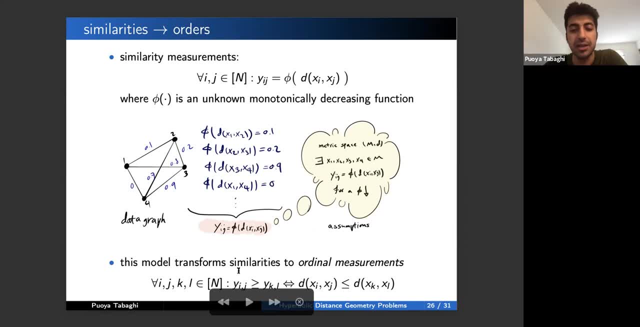 and we don't know what that is. the only way to interpret these similarities is that just to change them into ordinal or non-metric measurements. And that is like this: if what I said, like if i and j are more similar than k and l. 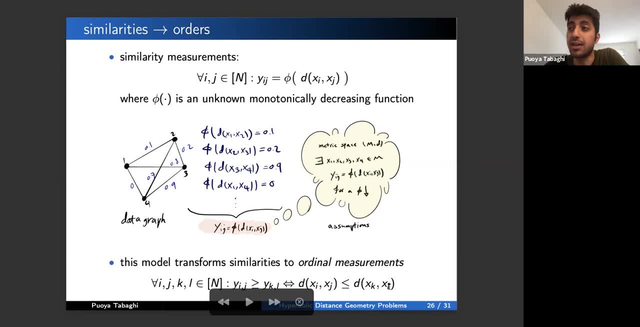 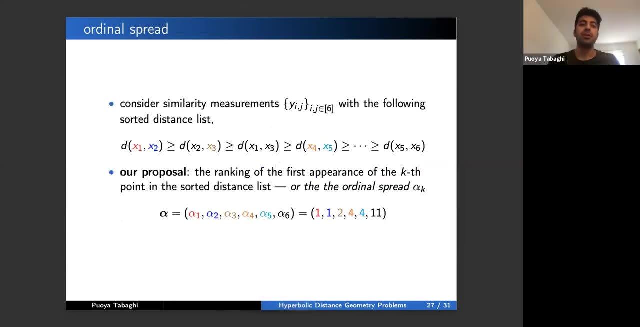 then xi and xj should be closer to each other than xk and xl. So these similarities are just as informative as these distance comparisons, just because phi is unknown and decreasing. Okay, so here's an example. Let's say we have similarity scores between six entities. 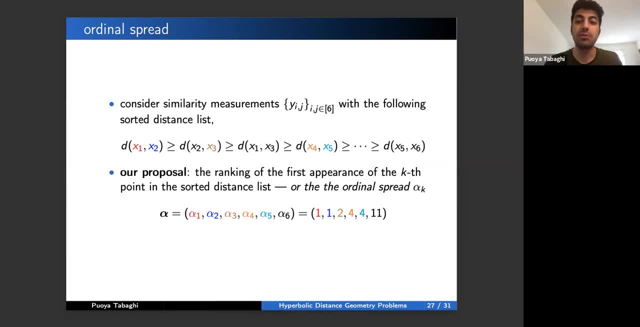 And so we know how to like transform these similarities into distance comparisons. So at the end of the day, I can get a sort of sort of distance list by just sorting these similarities right, And so I basically summarize these similarity measurements into a sorted distance list like this: 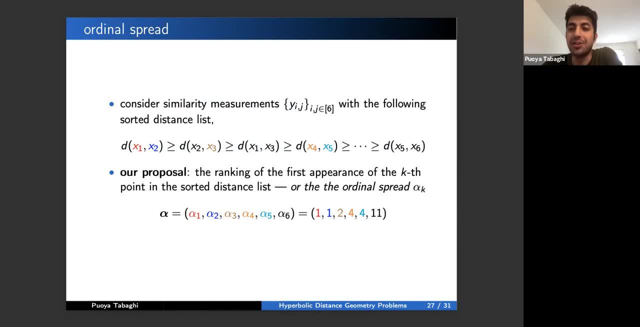 And I don't know what the underlying geometry is and I don't know what the distances are. basically, I just know these indices and the pattern of these indices, And the idea is to extract some features from these indices that are, that are indicative of the underlying geometry. 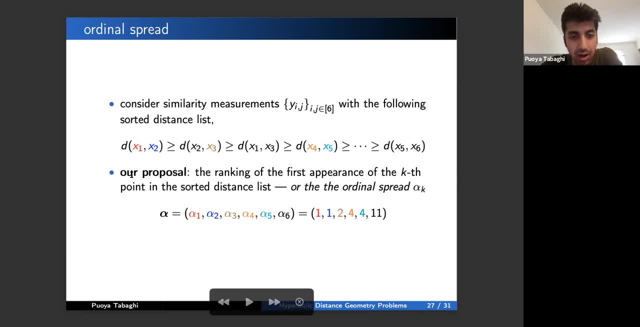 hopefully of these Xs. So our proposal is a notion called Ordinola Spread or Alpha K, And that is Alpha K basically is the ranking of the first appearance of the kth point in the sorted distance list. So I'm going to go through different case. 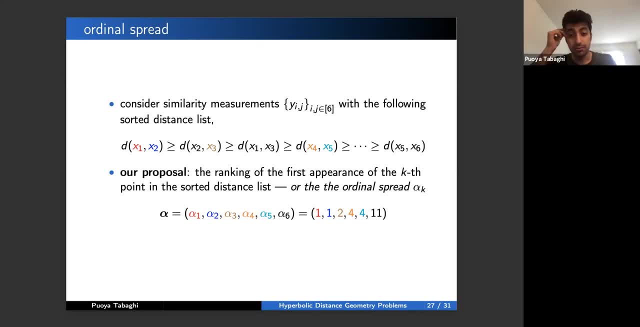 and I'm going to basically illustrate what it means. So Alpha one is the ranking of the first appearance of the kth. So Alpha two, Alpha three, They're going to be the ranking of the first appearance of the kth point in the sorted distance list. 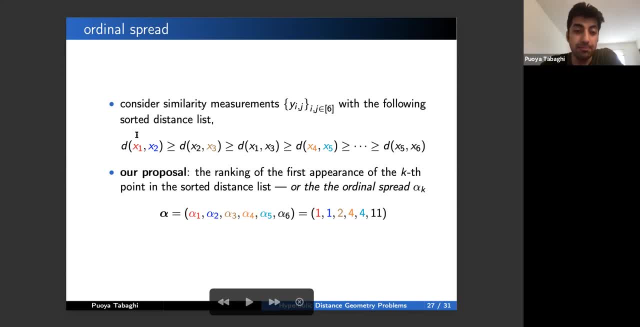 And then alpha three is the number of visits, for example for alpha two of the first point. So first point is X1 and its rank here is number one because it's the largest distance. So alpha one is one, And the second point appears for the first time here again. 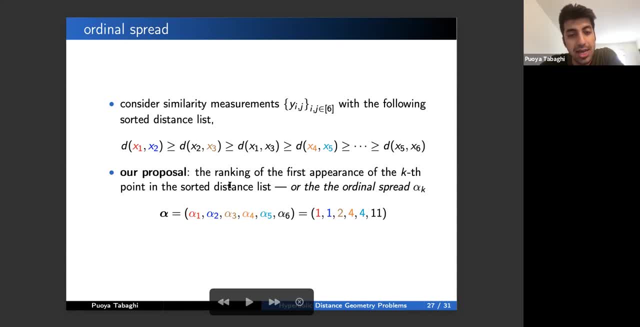 So its rank is also one, so one. And the third point is: X3 appears in the second rank, So there we go two. These two points have already appeared, so I'm gonna skip that. X4 is the fourth point that appears at rank four. 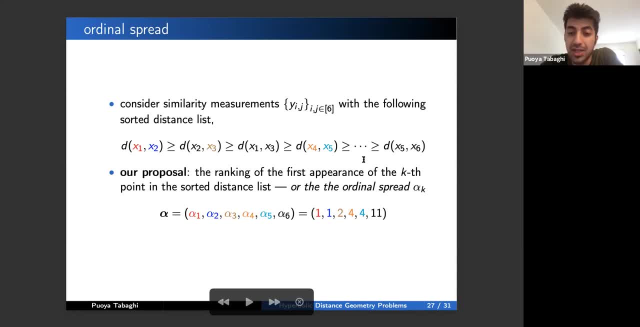 X5 is the fifth point and appears at rank four, And X6 basically appears, let's say, at 11th rank here. So I just derived the vector from these patterns, basically, And this is the ordinal spread vector, let's say okay. 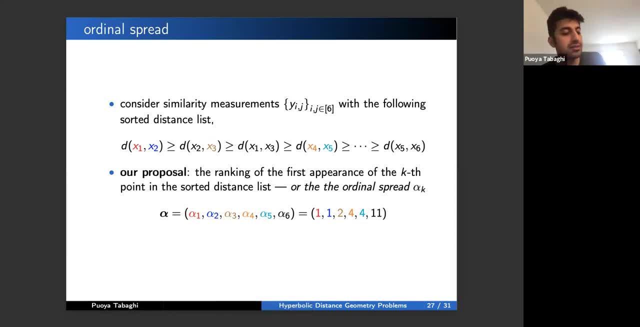 And there is some evidence to be to be had that the, basically the last index is quite important, Basically the ranking of the last point appearing in this distance list. So alpha capital N is important. So how do we use this in practice? We can have a data graph like this: 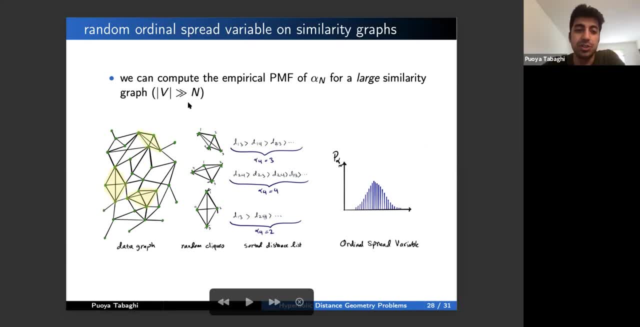 and we're gonna pick a number N, which is here like four, and we're gonna randomly select four cliques and then we're gonna have this graph. So here are random four cliques here, And because we have similarity of scores, then I have distance lists. 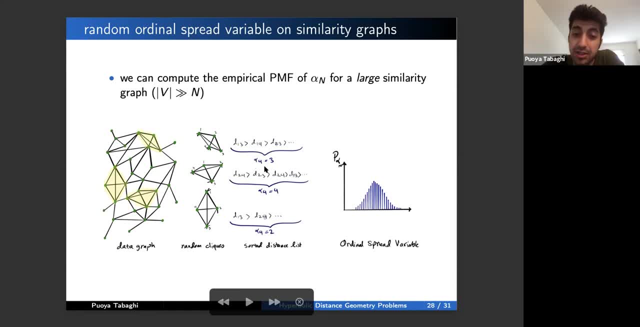 And because I have distance lists I can define, I can compute alpha capital N, which is here four. So here is three, here is four, here's two. And as I'm randomly generating these graphs, then I get random points like this: 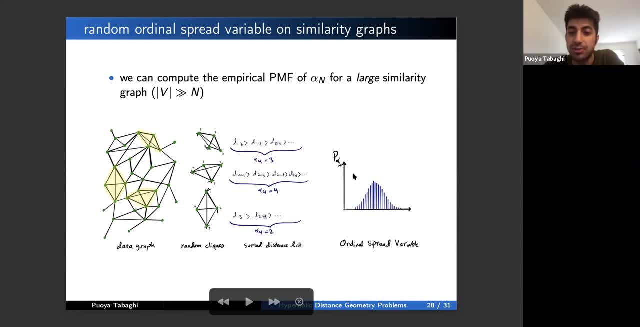 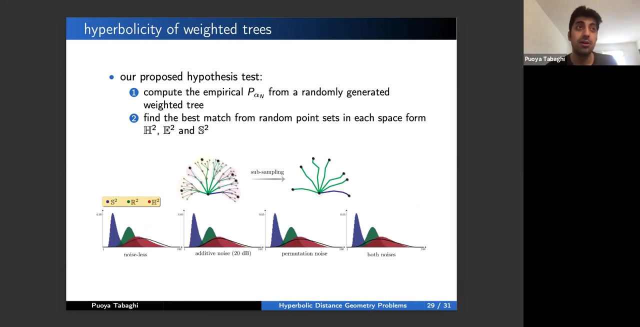 Then I can basically compute PMF of these random points. so I get to define a random variable on a data graph just by similarity scores. So this is going to be second to my last slide. So this is a simple experiment to showcase these alpha Ns do carry geometrical information. 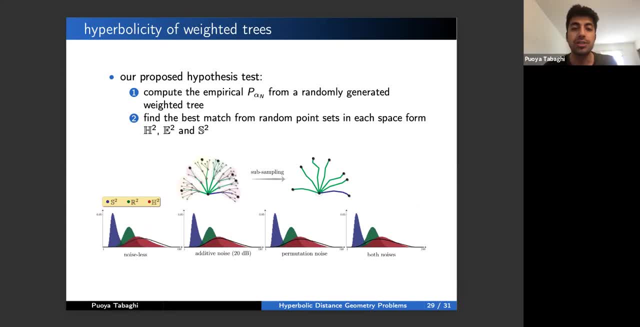 about the similarities. So here's the test. What we're gonna do is we're gonna generate a huge, huge weighted tree like this and we're gonna subsample it, as I just mentioned, and we get cliques like this. 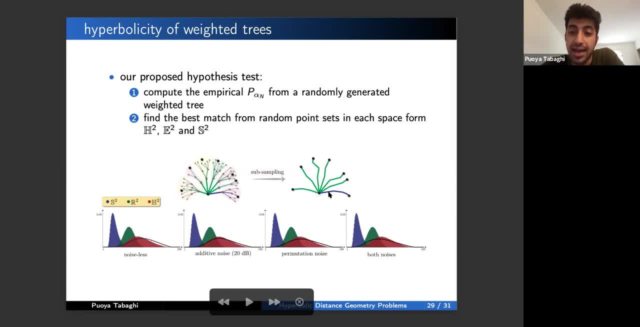 and we compute alpha N and it's PMF. So the PMF of alpha N is this black line here, right? And then I'm gonna propose a hypothesis test. I'm gonna say, okay, so this is the PMF, this is the PMF of alpha N for a weighted tree. 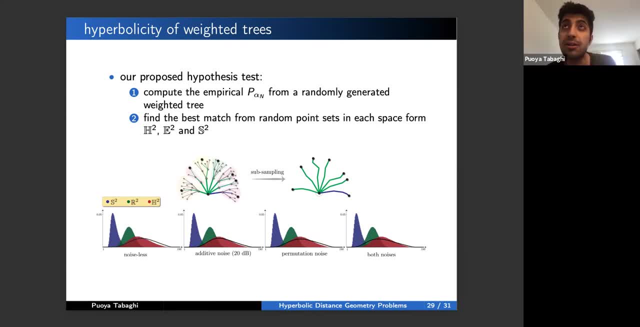 Should it resemble to random point sets in spherical, Euclidean or hyperbolic points sets. So I randomly generate points in each one of these spaces and I compute P of alpha N for each one of these spaces in like blue, green and red. 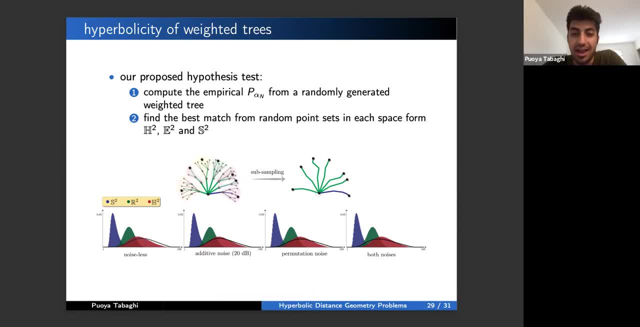 And I'm gonna do some sort of hypothesis test and almost in all cases- I'm gonna say almost in all cases, even with permutation noise and additive noise, it just the hypothesis test shows that the underlying geometry of a weighted tree should be hyperbolic space. 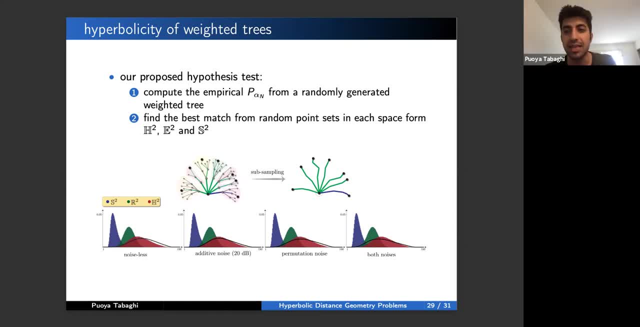 And that's just from distance comparisons alone. We didn't use any metric information, We didn't embed the data points, And so there's quite a bit of theory that goes along with this, but I'm gonna, just, I'm gonna just stop. 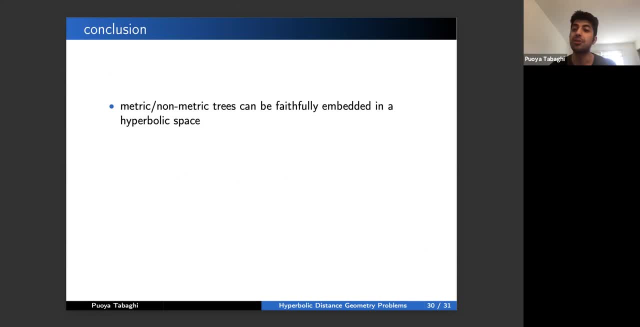 So, in conclusion, we showed the metric and non-metric trees can be faithfully embedded in a hyperbolic space. You propose a semi-definite relaxation to solve HDGPs and we show that hyperbolic for across this is almost identical to it's Euclidean version. 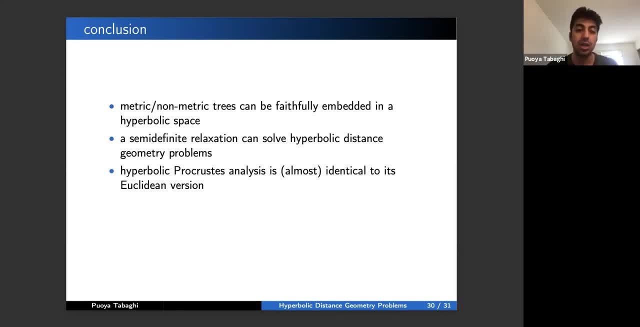 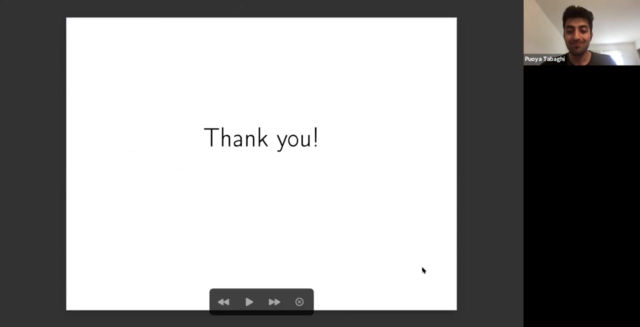 We have centering, we have central masses and translation rotations And also, finally, we showed that that there is a good chance that non-metric measurements can encode geometrical information about their underlying point sets. And thank you all. If you have any question, I don't know. 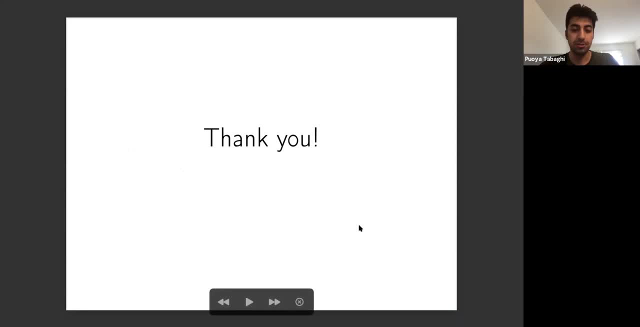 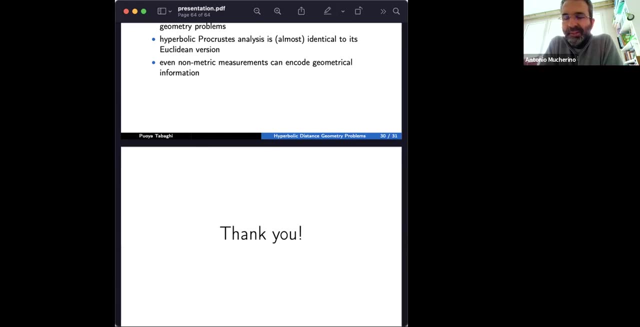 I didn't check if anybody had questions. Thank you very much. No, you don't have questions in the chat, but we have some minutes to see for the audience to react. Any questions from the audience? Just speak in case of questions. 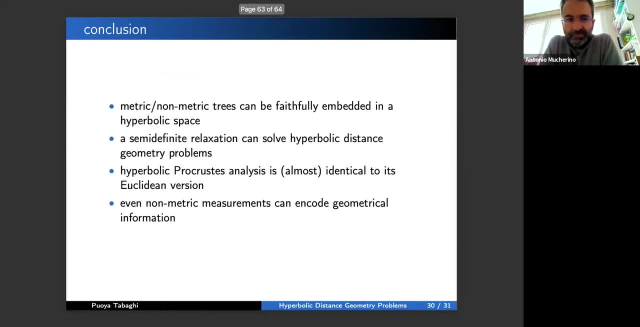 Hi Antonio, I have one. Yeah, please do that. Okay, Hi Pujoa. how I spell it? Pujoa, hi Pujoa. First of all, thanks for the very nice and interesting talk. I have a question concerning the applications. 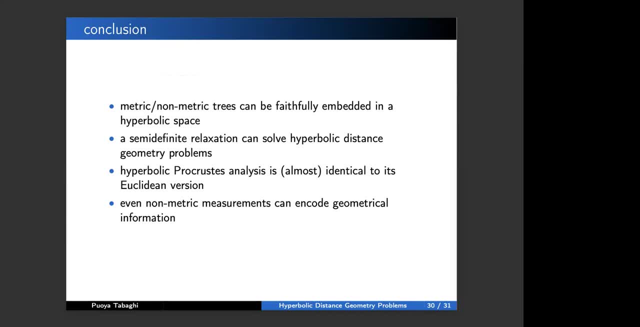 and also this, the third part of your talk, where you are discussing about the geometry of these similarity information, especially concerning the co-occurrences, For instance, in the natural language processing. it's a common problem to try to find word embeddings. 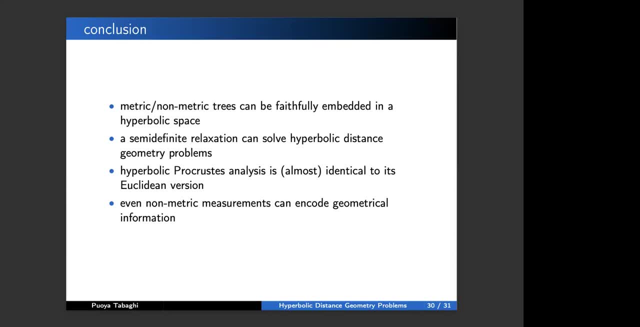 And I think in this workshop last Friday Sami Khalifi from Ecole Polytechnique gave a talk showing how we could use Euclidean geometry to try to find word embeddings. And I think in this workshop last Friday Samy Khalifi from Ecole Polytechnique gave a talk showing how we could use Euclidean geometry to try to find word embeddings. 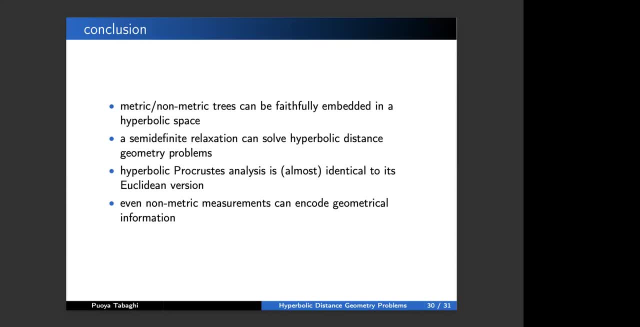 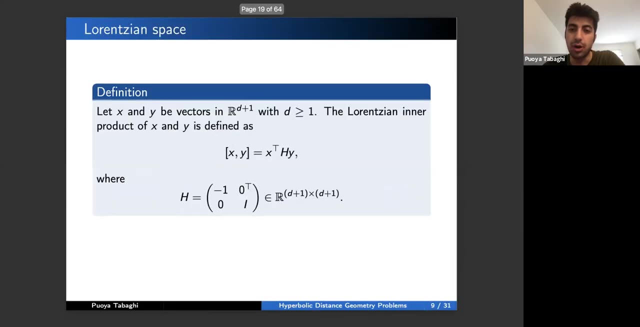 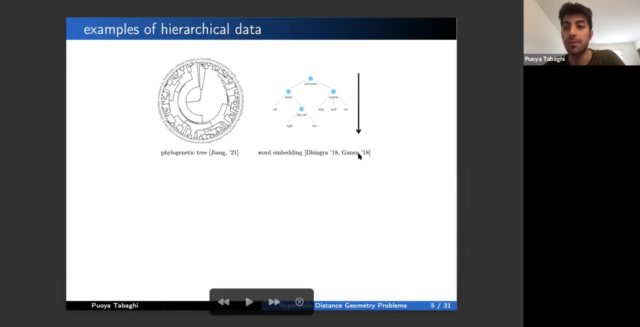 And I'd like to ask you if you are aware of any work using hyperbolic distance geometry to find these word embeddings and what could be the advantages? Yes, Okay, So there is this. these two works that I cited here, and they both use hyperbolic embedding for words. 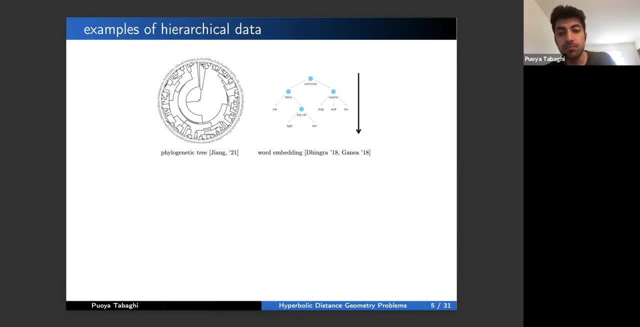 So basically Ghani especially, he proposed sort of machinery called like nested cones entailment to embed kind of hierarchical data And you have you measured like kind of pairwise hierarchy between nodes, And this is available in some word data sets like WordNet. 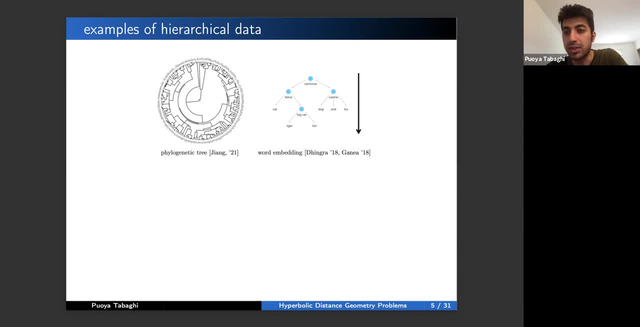 There are some semantic hierarchies that comes along with this database, And what embedding aims to do is to respect these hierarchical relationship between these points. And so, and then they would argue that this would give a better or more faithful representation if you use the same number of dimensions. 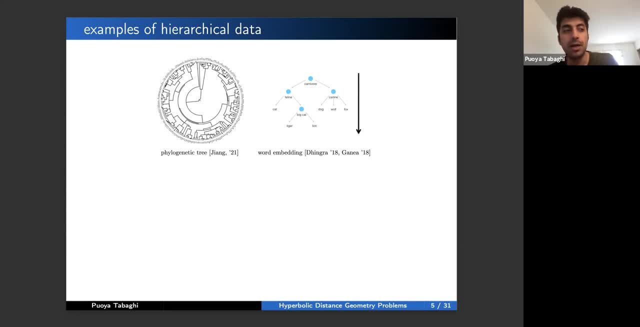 Actually, I'm not quite sure if they compare it with Euclidean, but the arguments is quite similar to what I just said, like that the trees can be faithfully represented in hyperbolic rather than Euclidean. It can be represent, they can be represented in Euclidean. 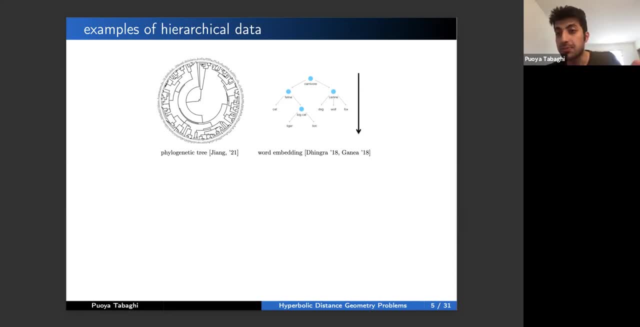 They just need exceedingly more embedding dimensions, basically. So that's a trade off. I don't know. Yes, Okay, Thank you. And concerning the co-occurrences, what are the differences? What do you think? I don't know if you already performed. 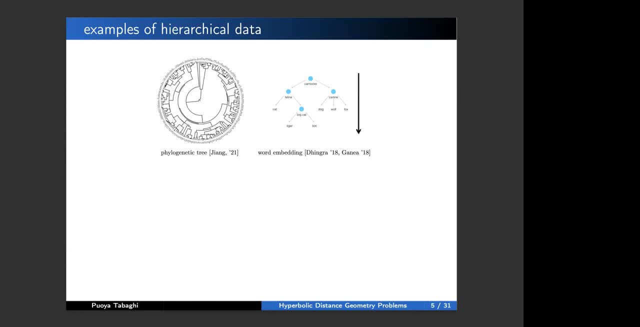 some experiments or not? What do you think is the correct geometry to try to model the co-occurrences? For instance, if you take the- I don't know- the entire Wikipedia, okay, And you count the co-occurrences of window. 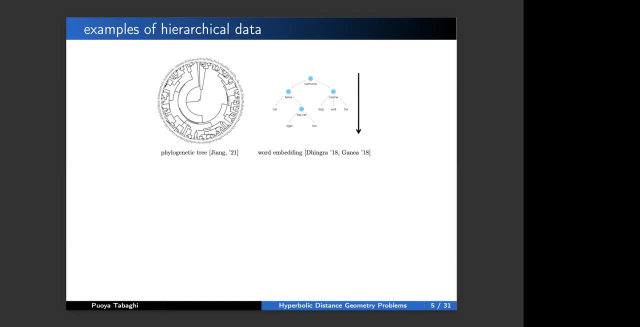 of words occurring in a window of a certain size. okay, So this co-occurrence, information or similarity could be more- how can I say better, represented by which kind of geometry? I'm not quite sure about co-occurrences specifically. 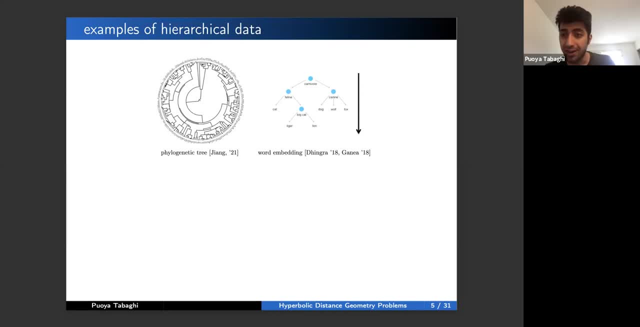 but we use some other metric to define similarities. It's called relative forest accessibility. It is another notion of similarities And what we got for our data set, which was like single set RNA sequencing data, it was a spherical. We found this spherical to be the 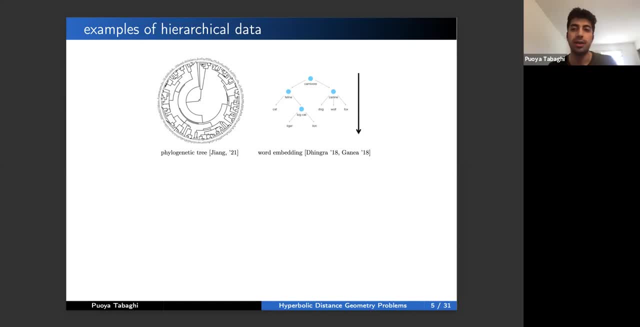 optimal embedding measure. Actually I have some results, but I didn't put it in is a slight, So I think you just have to run this analysis like this, or you know, spread and stuff, to give you a hint a little bit that, like you, would get a curve basically. 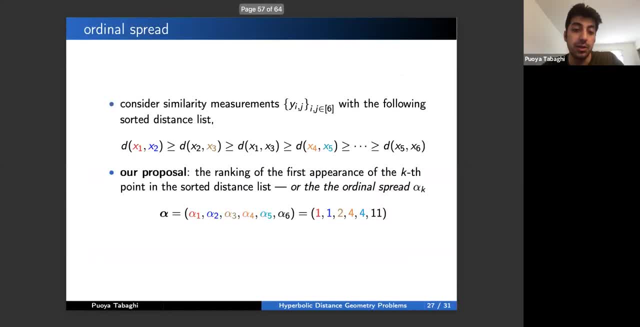 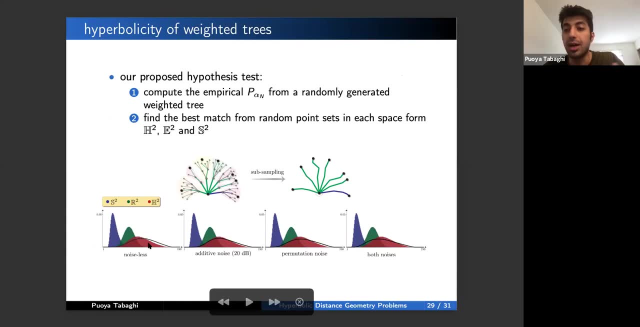 if you implement the algorithm, that basically will lie somewhere between this blue, green and hyperbolic, and then that would kind of give you, give you an intuition which is based. it can be best that be embedded in. okay, thank you for the hint. any other questions we have time for.